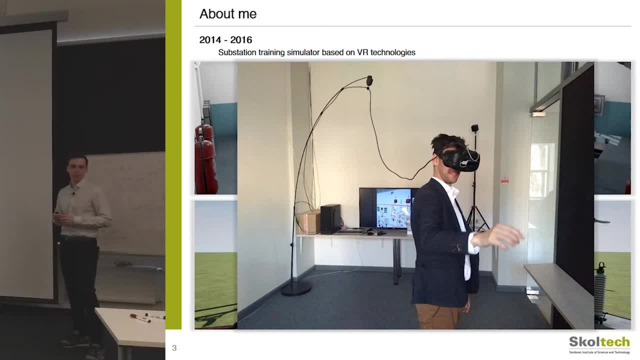 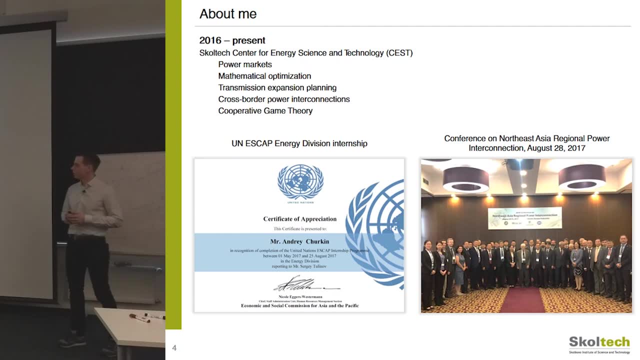 David enjoy it. So if you're interested, approach me and I can tell you the name of professor and you can visit this simulator. And in 2016 I joined Skoltech and I completely changed my topic. I started studying power markets, mathematical optimization, transmission, expansion, planning and in 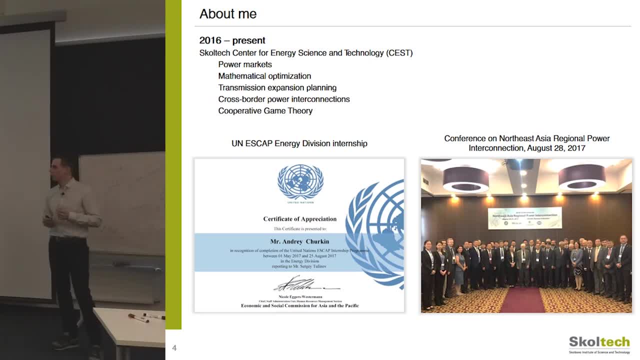 particular cross-border cooperation And in my during my first year I had a chance to undergo an internship in United Nations in Bangkok and also participate in the United Nations conference in Irkutsk, And after that I realized that there is a strong political and. 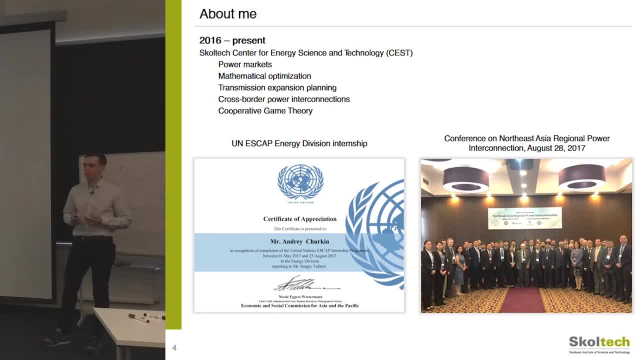 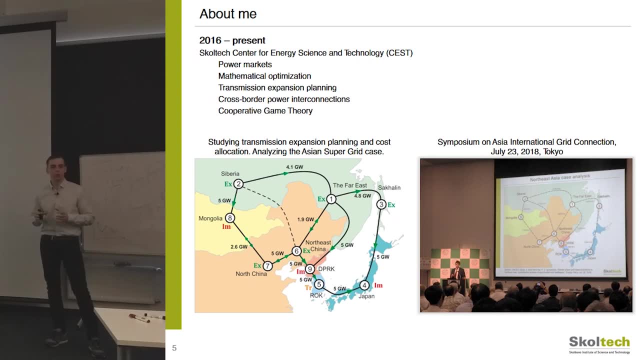 economic interest in cross-border electricity trade And therefore we started running transmission expansion planning for the for some cases, For example for the Asian super grid case, and also I was invited to the symposium on Asia international grid connections in Tokyo And after that we finally 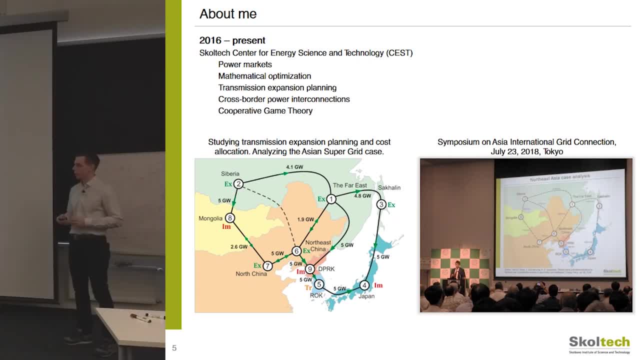 decided that this will be the topic of my thesis. But the question raised: what new can we do here, How to bring scientific novelty? And after several discussions we realized that there is a need to use cooperative game theory in order to allocate the investment costs of such projects among the countries. 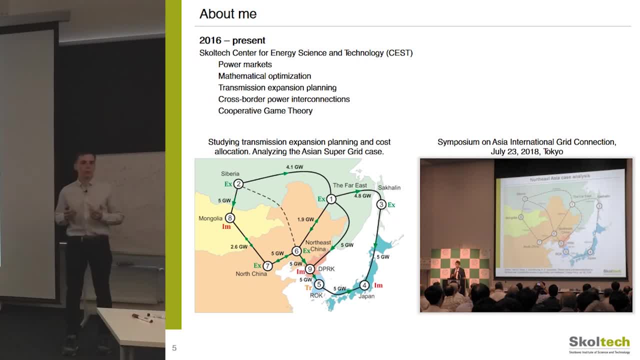 Because before this the usual question was how to optimize the interconnections, how to make this cooperation optimal. But very few papers address the issues of cost allocation. And also I want to highlight that there are many projects of power interconnections in the world, especially in Europe, in the United 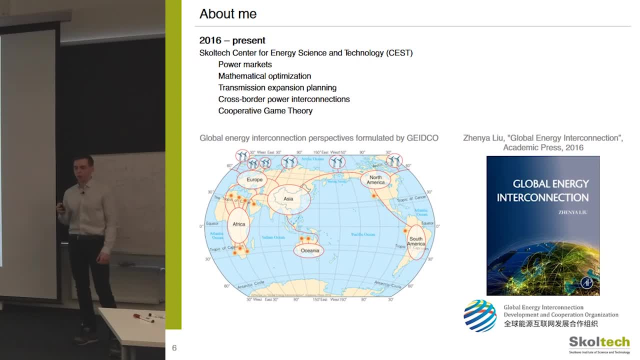 States in Europe and in North America, And one of the greatest organizations that exist so far is called Global Energy Interconnection Development and Cooperation Organization. that is created by Chinese state grid corporation And they are developing huge plans like cross-continental power interconnections. 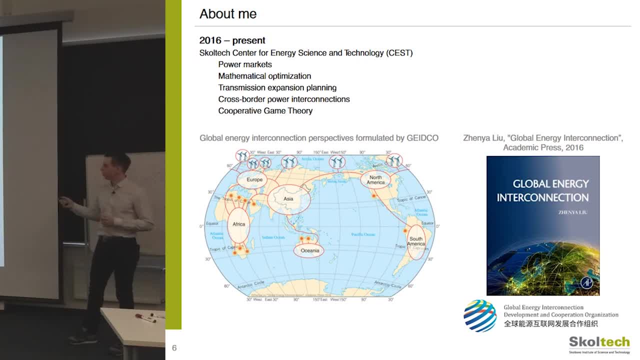 And, by the way, I think that we still have several copies of this book by Liu Zhenya and if you're interested, you can approach me or David and we will share it with you, But it is in Russian, So, as I said, we understand. 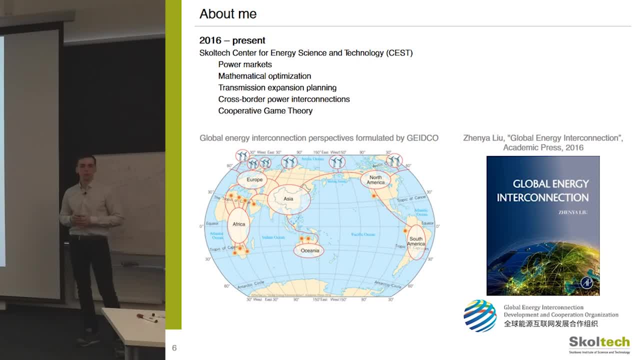 in Scottish dialogue. no, it is translated to Russian and Chinese company granted it to us, But you can find an English copy in the internet, I think. So, yes, after this preliminary research, we realized that there is a need for cost allocation techniques And also, as you, 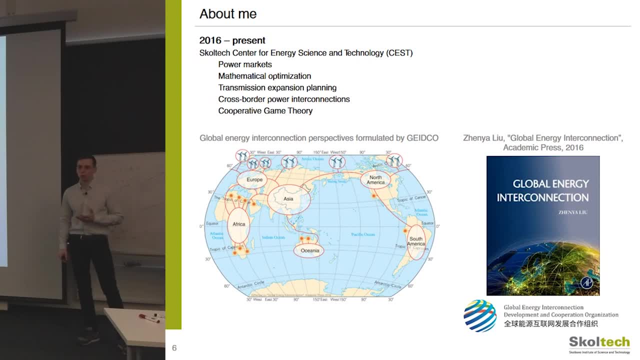 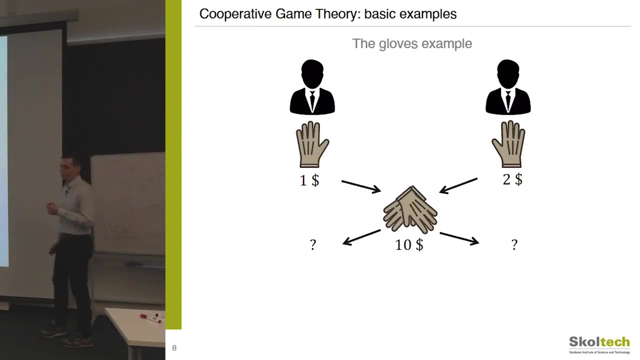 may see, three years ago I knew nothing about cooperation game theory. I had to start from scratch, and therefore today I want to show you how my research evolved and motivate you to use the same techniques in your studies. so let's start with my favorite example, one of the simplest ones, that is. 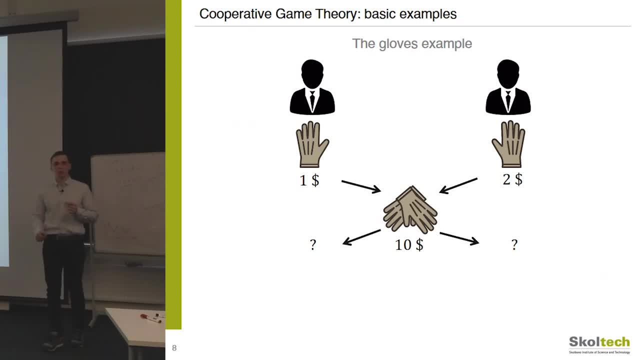 called the gloves example, and I would ask you to imagine that you are the left person that has the left glove and this glove is not of such a good quality and you know that you can go to a market and sell it for one dollar, but you have. 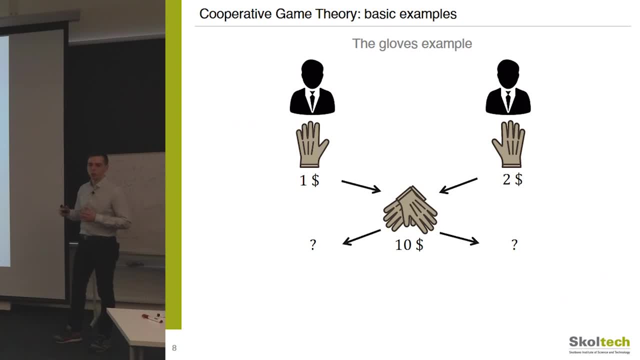 another person that has the right glove, that is somewhat better, and you know that. and he knows that he can sell it at least for two dollars. but if these people cooperate and they make a pair of gloves, they together can get ten dollars. so this is an example of mutually beneficial cooperation, and the only 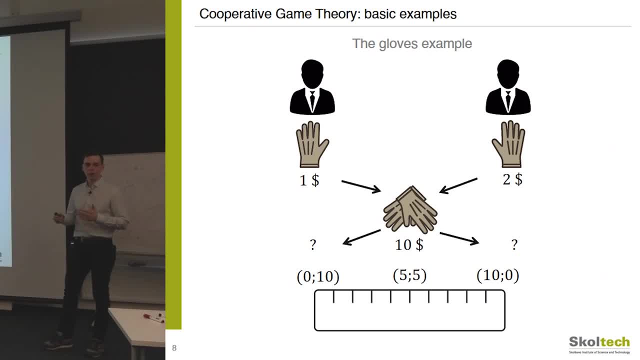 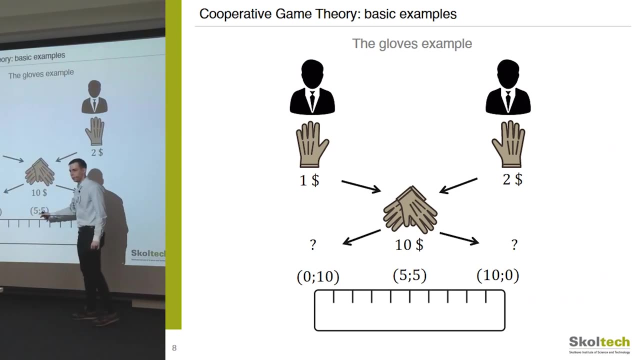 issue is how they should split the ten dollars among themselves, and this is the question that I want to ask you, and in order to help you, I drew here this empty ruler and you may see the points like zero- ten. this means that you get zero dollars, another player get ten dollars, the half division and ten. 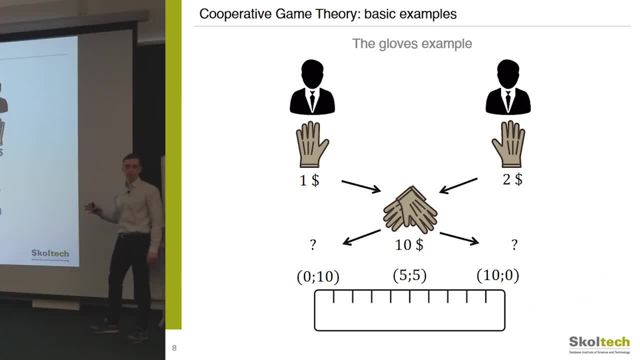 zero. so do you have any ideas how you can split the ten dollars proportional to initial cost? it is, it is, I would say, semi correct, because it is possible to do. but but what if one glove will cost very close to zero and then the proportion will be huge and, and this, this, this could. 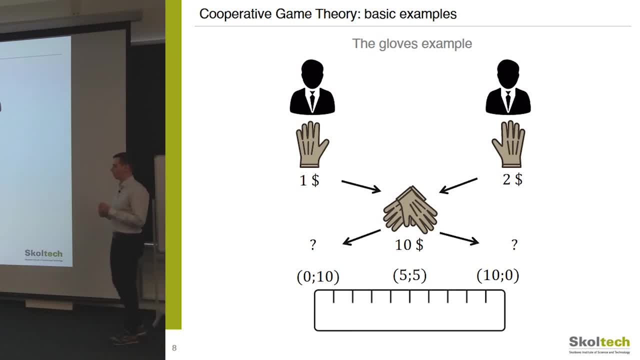 lead to some strange results. and in order to give you some ideas, let's consider: is it possible to find a solution here like ten dollars zero at this point at the end of the ruler? did you ask this question to you, this exact now? no, but but. but I remember. I. 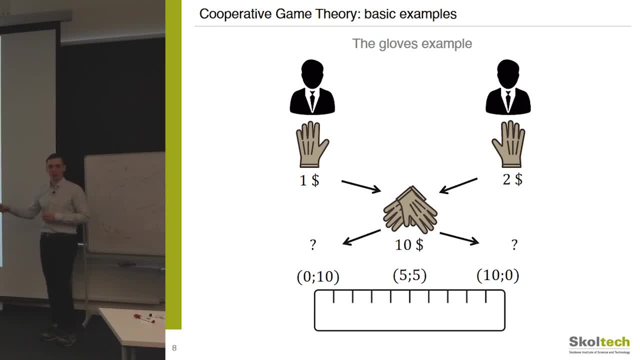 just can't resist to ask this question. I remember at INFORMS conference I was talking about this And Yuri passed by and he looked and then he just continued walking. So probably he didn't like it. Oh no, he wouldn't miss that. 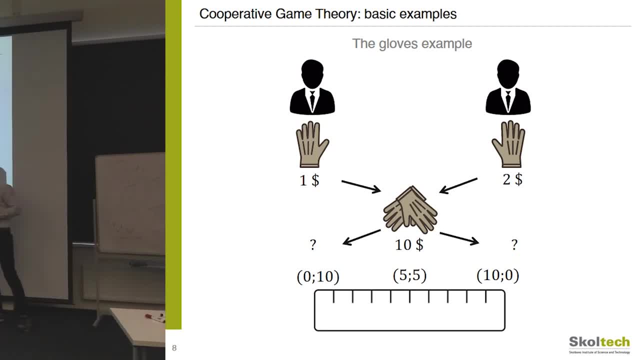 OK, so if we consider a point, $10 to one person, $0 to another, this is an infeasible point because it's not rational. The player can get $2 on his own And by this simple logic we can understand. 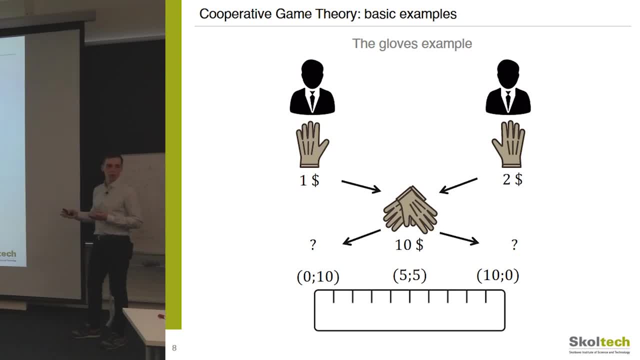 one of the basic cooperative game theory concepts that is called the core of the game And we can plot it on this ruler, the green space, the feasible solutions to this problem. And through this lecture I want to show you that, even though cooperative game theory may, 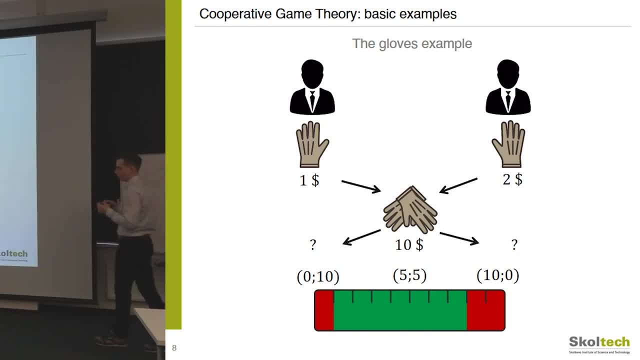 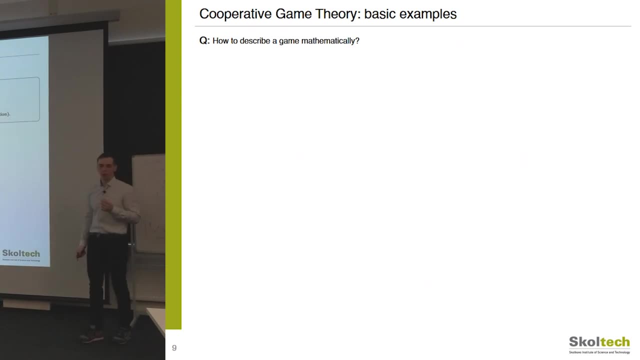 seem a bit complicated. it is based on very simple, intuitive concepts that you can realize, in a few months, maybe. And OK, how can we solve this problem mathematically? And the answer here is that we need to describe all possible coalitions. 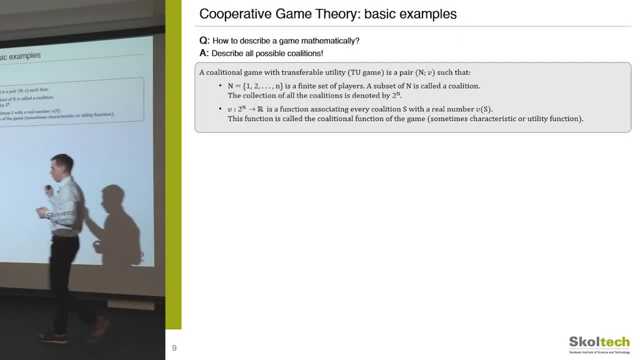 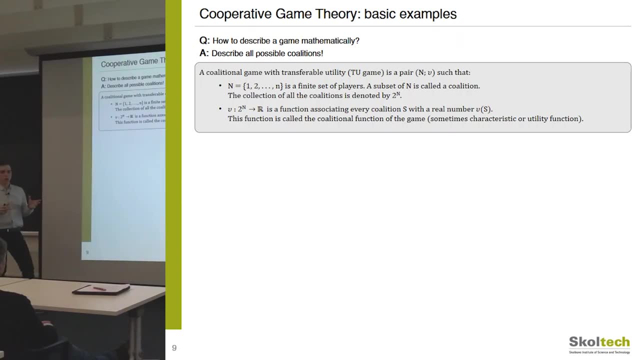 And I will give several simple definitions here. The first one is that we need to know that we have a set of players and a set of coalitions. The main concept is that we need to describe two things. First is a set of players and set of coalitions. 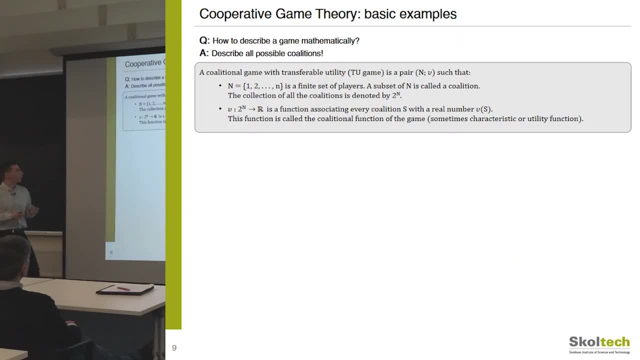 what coalitions we have and what players belong to them. This is like a combination of possible scenarios, And the second is the so-called characteristic function, new. that describes each of the possible coalitions, And once we describe this, we can also. 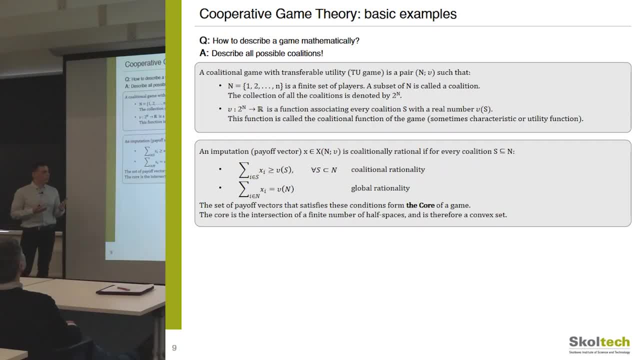 formulate this rationality concept, that is two basic conditions, And the first one is called a coalitional rationality. This means that each coalition cannot get less than it gets on its own, And this is what we see. If you have $1 for your left, glove. 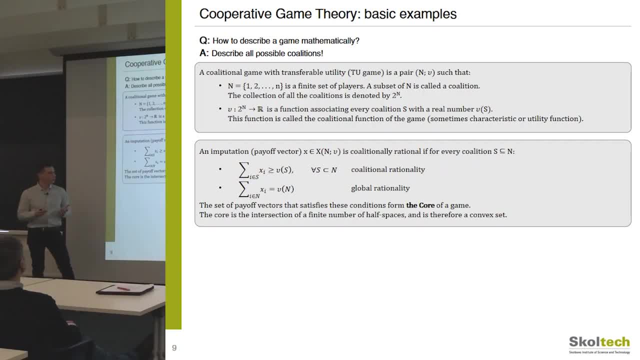 you will not agree to get less, And the global rationality constraint means that the gain of all of the grand coalition should be equal to the payoffs of this coalition. So we keep these allocations And if you have $1,, $2,, $3,, $4,, $5,, $6,, $7,, $8,, $9,, $10,, $11,, $12, $13, $14,, $15,, $16,, $17,, $18,, $19,, $20,, $21,, $22,, $23,, $24,, $25,, $26,, $27,, $28,, $29,, $30,, $31,, $32,, $33,, $34,, $35, $36,. $36,, $37,, $38,, $39,, $40,, $41,, $42,, $44,, $45,, $46,, $47,, $49,, $50,, $50,000, and $60,, $52,, $53, and $54, is greater than $2. 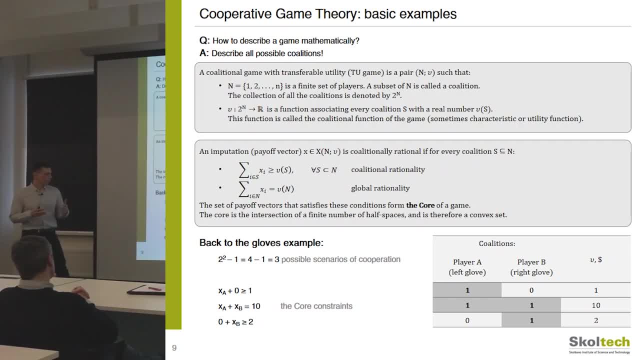 And you see that this is pretty simple and easily programmable And, moreover, the core is formed of these hyperplanes And therefore it is a compact convex set And you can perform any additional optimization or any additional techniques within this set. 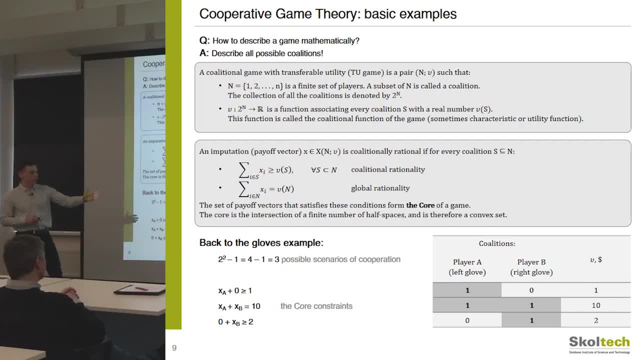 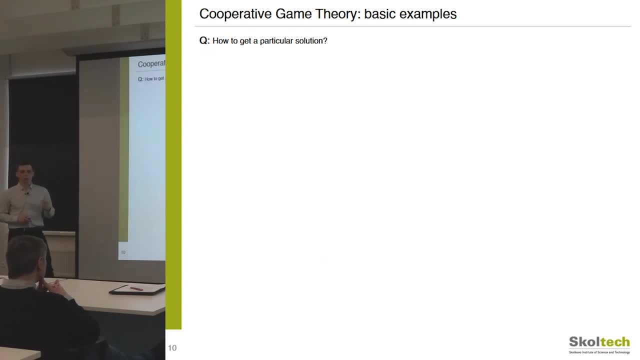 And also I drew this table for you, when you see what are the coalitions, the three possible coalitions and their characteristic function, And the next question that you may ask, but how to get a particular solution for the problem, And the answer is that there is no single solution. 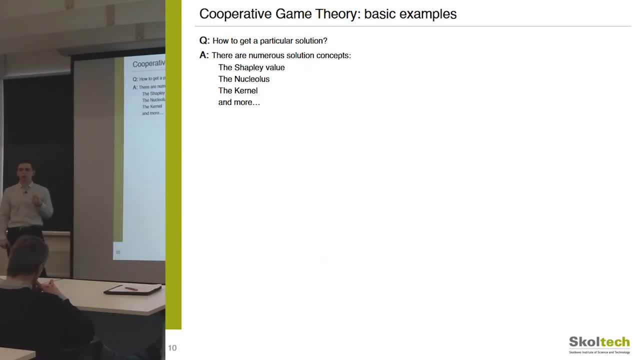 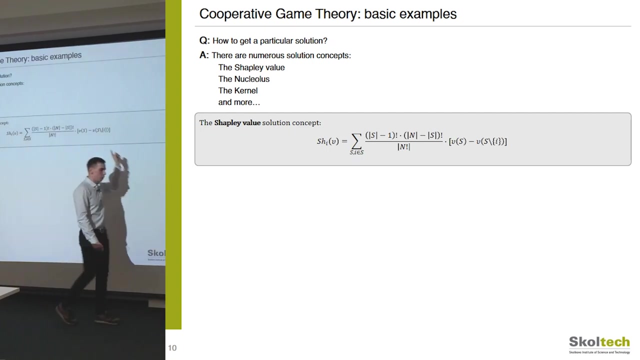 There are many solution concepts and the most famous one are the Shapley value, the nucleolus and the kernel. And let me introduce the Shapley value. that's probably you heard about. The formula may seem complicated to you, but first let's talk about this right component. 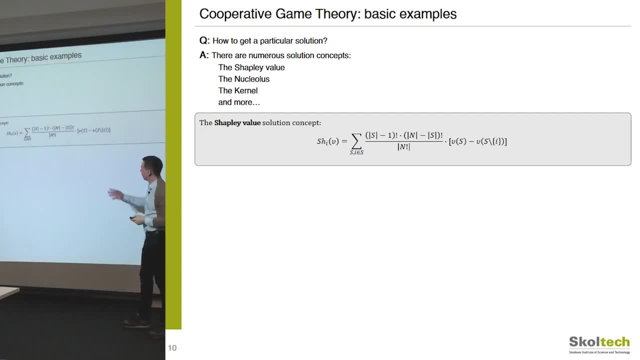 And this is called the marginal contribution of a player to a coalition. This is the difference between what coalition gets with the player and minus what coalition gets without the player. So this is like a margin of what player brings to a coalition. And in order to better explain you this concept of marginal contributions, I heard a rather 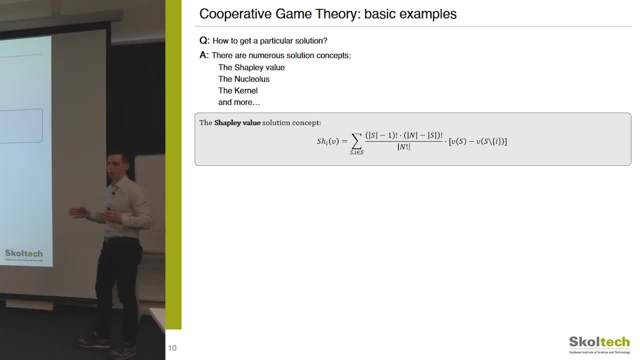 funny example. You may imagine that there is a room and several men entering it And the goal is to lift something heavy. And let's see what are the marginal contributions. If the first man comes, He tries to To lift a heavy weight and he achieves nothing like zero result. 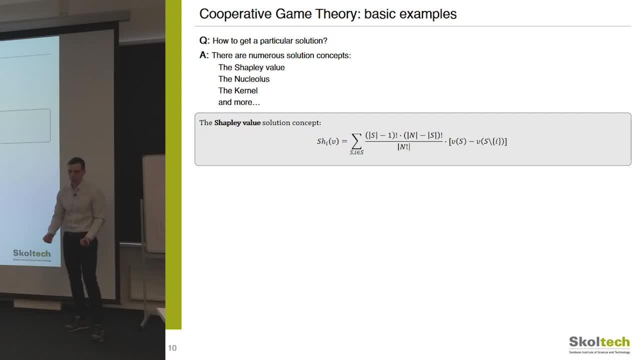 And then more and more men are coming And finally the last man helps and they lift this heavy weight up And if we consider marginal contributions, they will be like zero, zero, some small contributions and a huge contribution. So this very smart formula by Shapley: it says that we need to consider all possible. 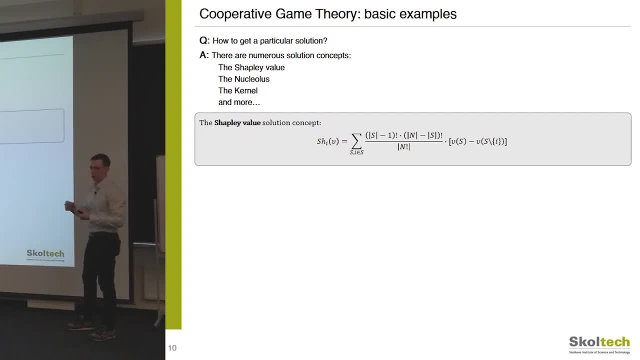 contributions, all players to coalitions in all possible orders. So we need to consider How the man can enter the room in different orders and lift this up, and then to allocate this gain to analyze the effectiveness of each man, And we can do this for the two gloves, example. 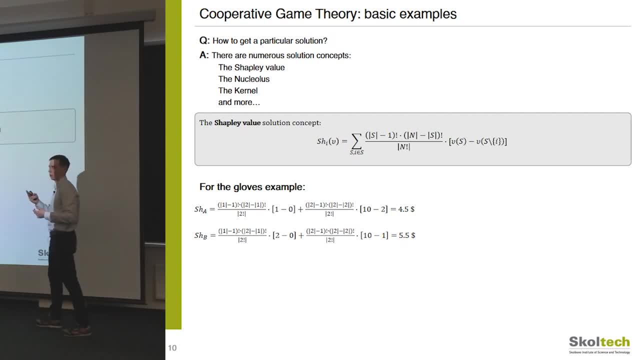 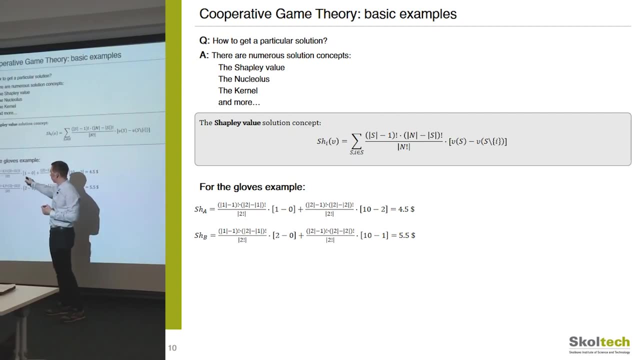 And this is rather easy. We can calculate it here manually, because there are only two scenarios: They cooperate or they do not, And we see that this is coalition of player one with the left glove minus zero, because there is no cooperation at all, And the grand coalition minus. 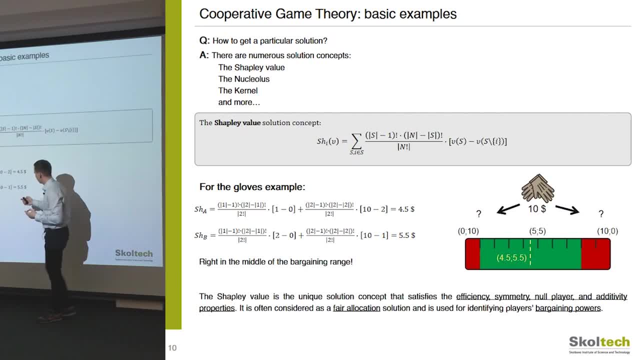 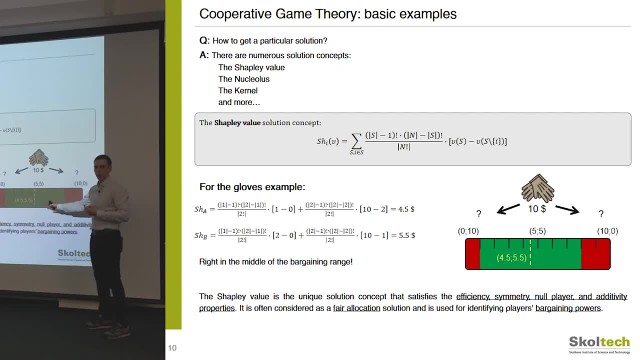 Minus The grand coalition, without player one, And in this fashion we get this interesting result for the five and five and the five. And this is right in the middle of this bargaining range, And this makes sense to me because you see that players in this cooperation they have 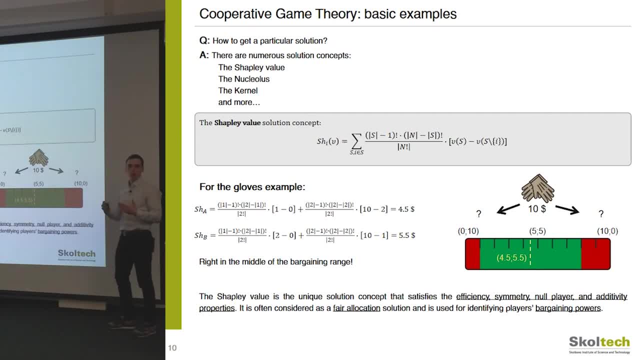 equal bargaining power, equal influence, They, both of them, can break the agreement And therefore this surplus is divided by half. And yes, So it's somewhat counterintuitive because the ratio of these coalitions. So it's somewhat counterintuitive because the ratio of these coalitions. 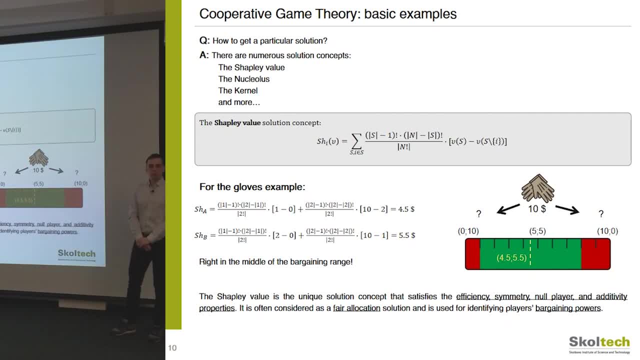 And therefore this surplus is divided by half, And therefore this surplus is decorated by half, And therefore this surplus is decorated by half Of this course- is not 2 to 1 as you image it- And therefore this surplus is decorated by half. 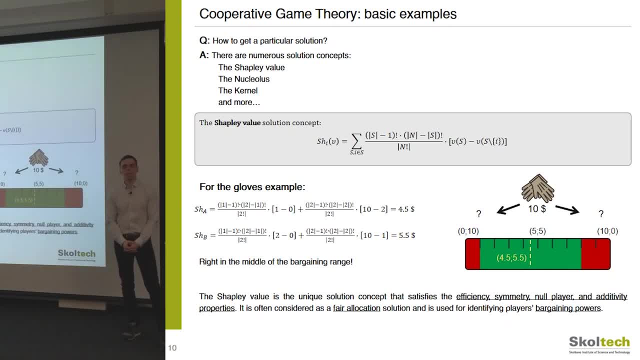 Because someone kids: well, you can go what you want. you should buy this in the store. There is no time in the store, There is no money there. the man: You can go what you want, But sometimes you can go in here, but it goes Russian. 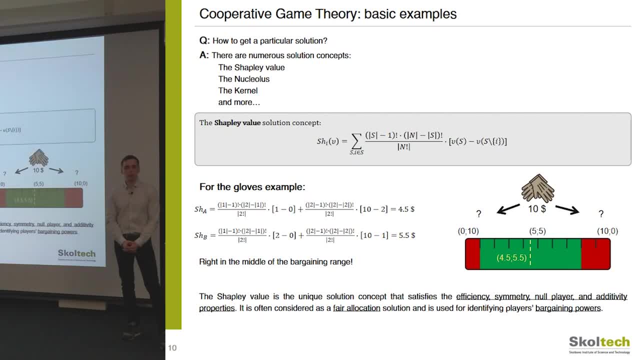 And, yes, you should divide this 10 by like: three goes to the right and one to the left, according to the yes, this is the ratio, which actually this is not the ratio approach, And you see an interesting fact, that the difference between the left and the right glove was $1.. 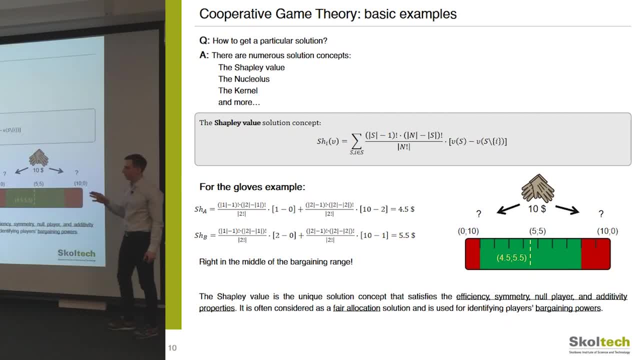 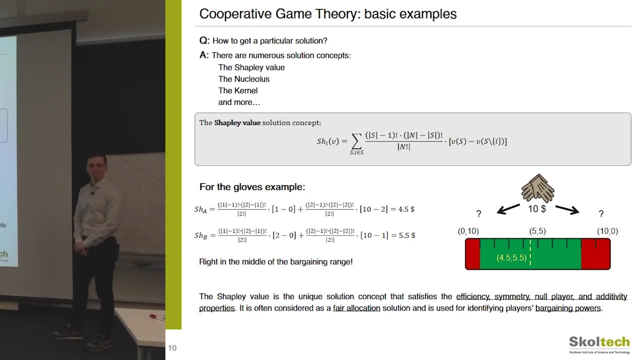 And this difference preserves it here. So, but this is a simple example And therefore we get such a simple solution And Shapley uh uh, often referred as the efficient and fair uh cost allocation. just, yes, sorry, just just one question, because it could be related to practice. suppose you have not such a good glove in the 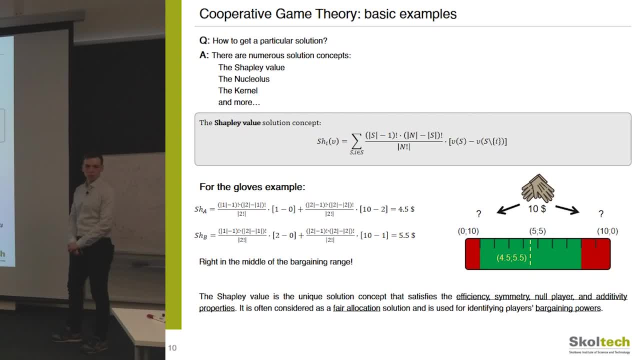 right hand part. suppose you have a glove that, for example, costs one dollar. yes, and you're about to make a decision on investment in its repair. yes, so that it costs more on its own. but then when you plan that you're going to have a coalition, maybe you won't make this decision on investments in. 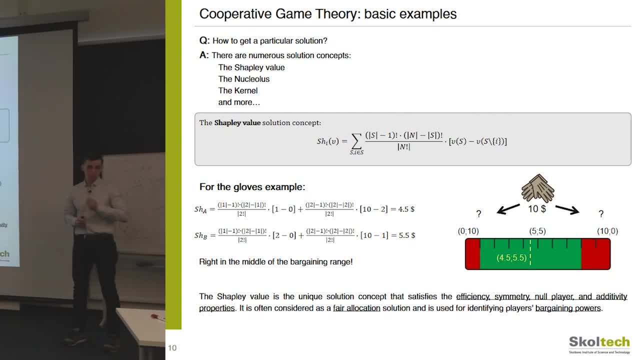 repair. in other words, it's it's related to power systems, because you can measure these shares of different participants in terms of, i don't know, complexity of their infrastructure and then when they combine together, if they plan that ahead, they might affect severely their decision, investment decisions. therefore, we assume perfect information, if not perfect information. 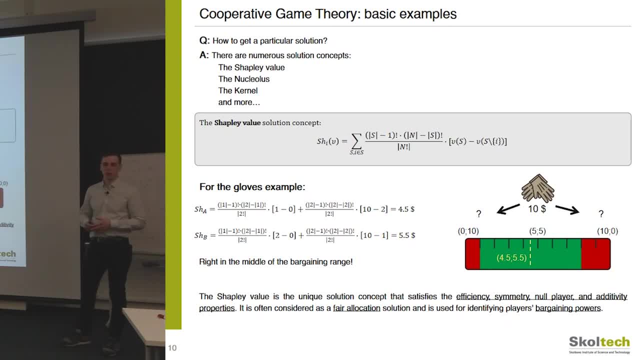 then the players could cheat, they could say: my glove is infinitely good, okay, okay. and this is the simple example, and because of these properties and this uh account of marginal contributions, the shapley value is often called as the fair allocation concept and it is used to measure a player's bargaining power. and let's see the similar example, but in power. 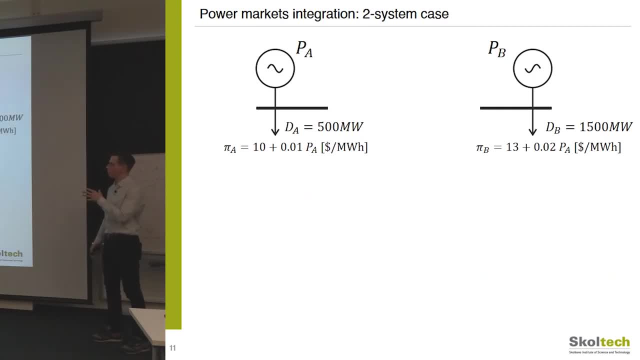 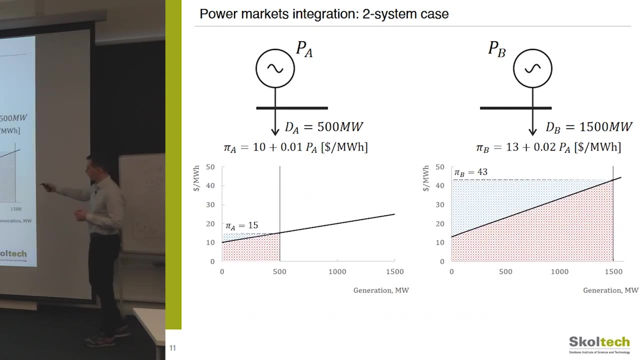 systems. imagine that there are two nodes with certain demand and generation, and we can set the generation cost functions and you may notice that cost function at power system b is higher. we can plot this and see that indeed the generation costs this red area in system b is. 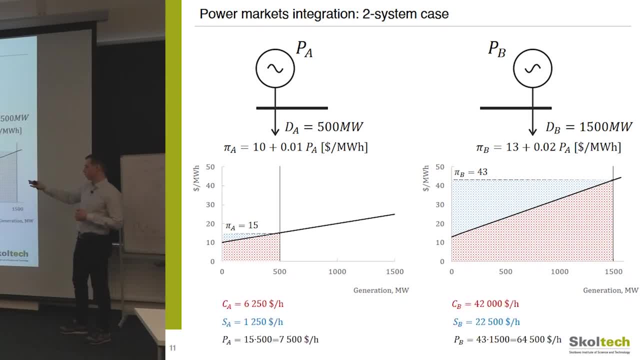 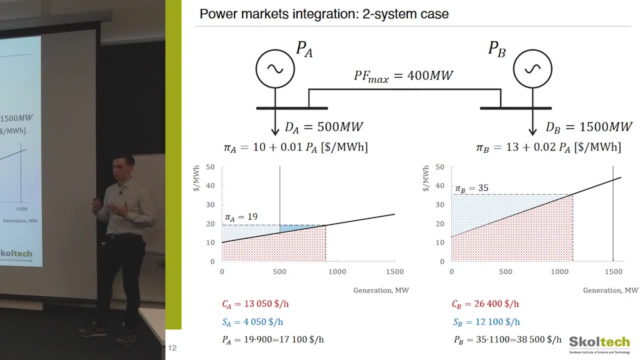 much higher and this blue area is called the revenue of generation companies, so we can call this the social welfare. and if the countries agree to build a line, let's say 400 megawatts, we can see how the situation changed. there there occurs, there is now a power export from system 8. 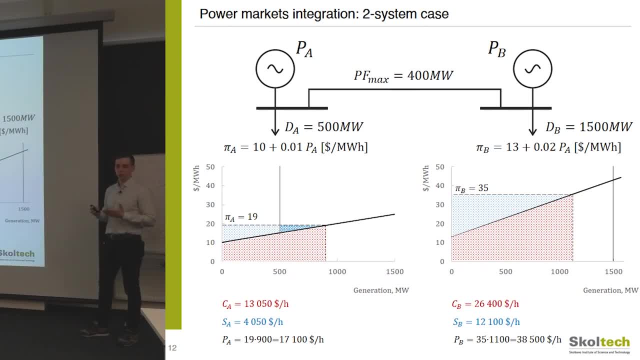 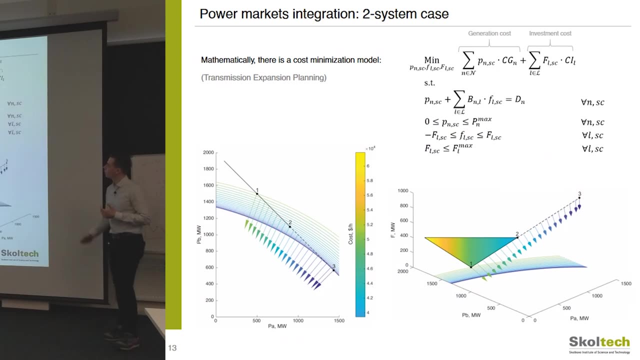 b and the overall generation cost decreased. and also from the mathematical point of view, this problem is similar to power flow optimization or transmission expansion planning, where in the objective function we see the minimization of generation costs and investment costs. but in this simple example i created not a constant- not a constant uh generation cost, but a linear. 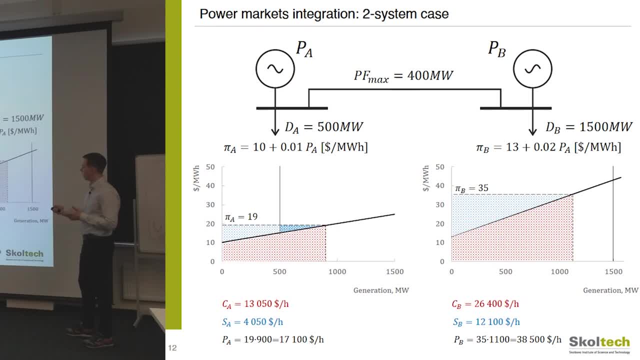 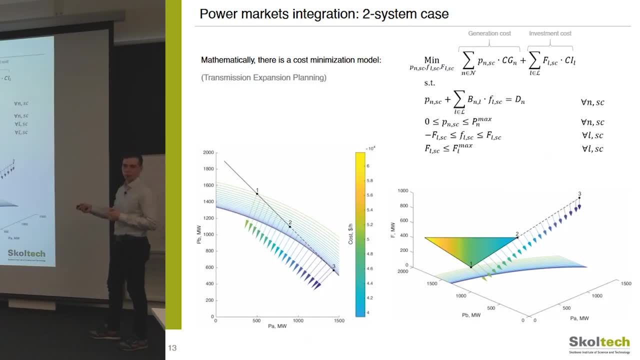 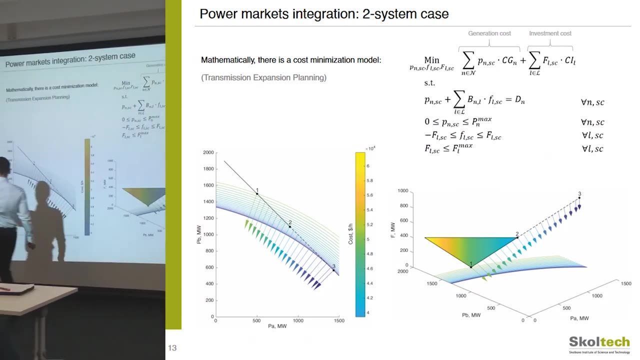 function and therefore the cost itself is a, an integral under the function and it is a quadratic function and therefore in these pictures you may see that this, it is a quadratic optimization and this is the power generated by the expensive generators in power system b, in power system a. 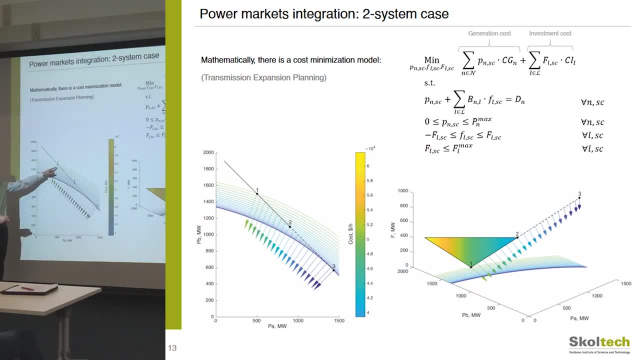 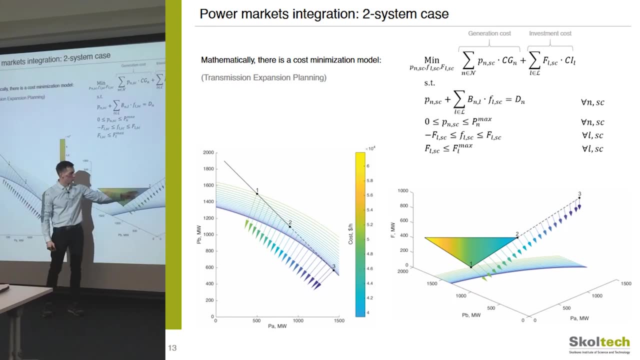 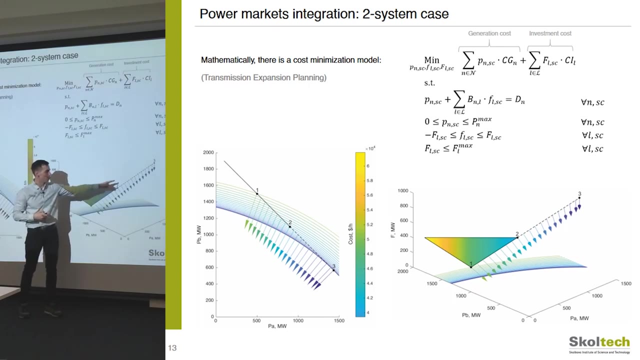 and the initial point one, when there is no cooperation, and this is the 3d figure. so once we build more capacity, this space evolves here and we come right to the point two, the most, uh, the least cost point for the system. we can go even further, to 0.3. 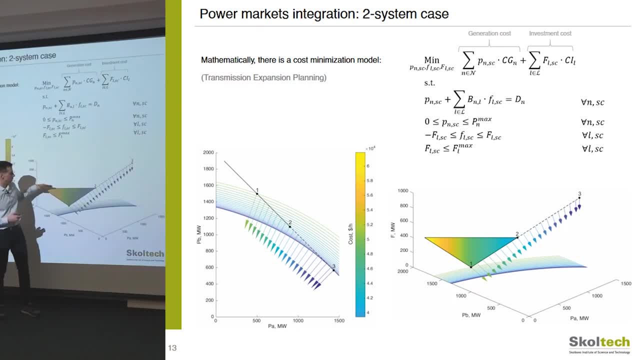 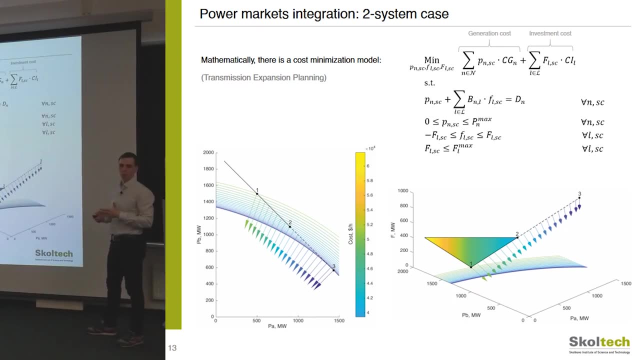 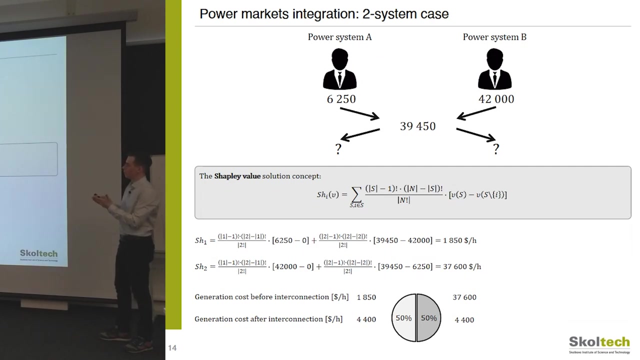 but it's impossible because there is a restriction on power capacity and if you consider, yes, we say 400 megawatts maximum, and they achieve this. so point 2 is the feasible, optimal point. and coming back to cooperation, we say we see the same players, system A and system B. they had some costs before and some costs together. that 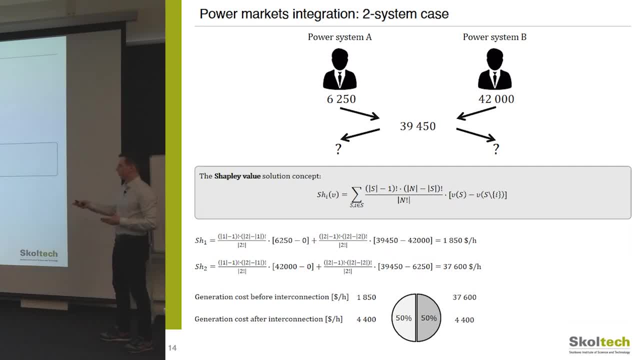 is decreased. We again can calculate this simple Shapley and again see the generation cost allocation by the Shapley. And even though these values can tell you not so much, you may compare them with the initial costs like separate costs of no cooperation and you may see that the savings are allocated. 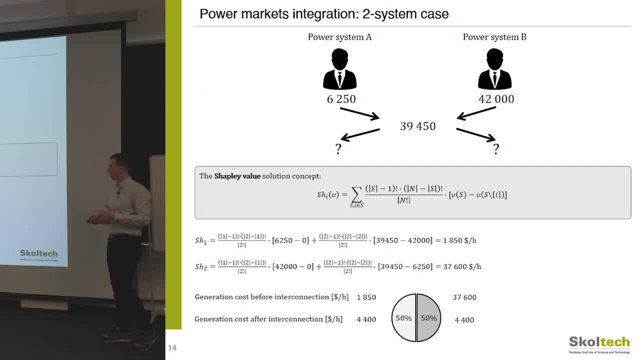 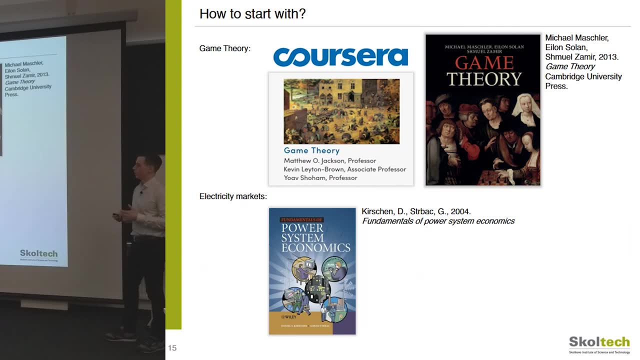 equally again, And this is the fair solution for the problem. And yes, as I said, I started studying cooperative game theory principles from scratch and I want to share with you just some ideas how you can also understand this. First of all, I watched the course on Coursera introduction to game theory by Matthew Jackson. 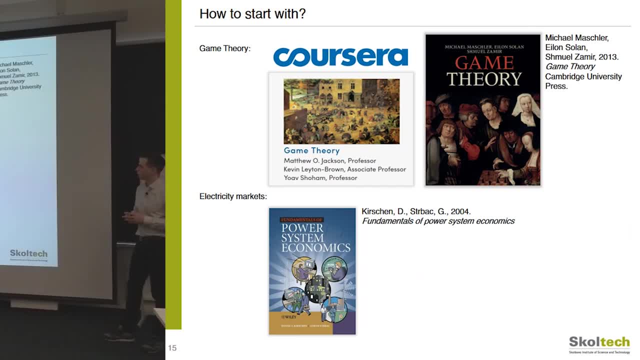 It was very useful and encouraging And, once you understand basic concepts, I recommend you this famous book by Michael Maschler about the game theory, and it describes both non-cooperative and cooperative game theory concepts And about electricity markets, operation and economics. I think most of you know this. 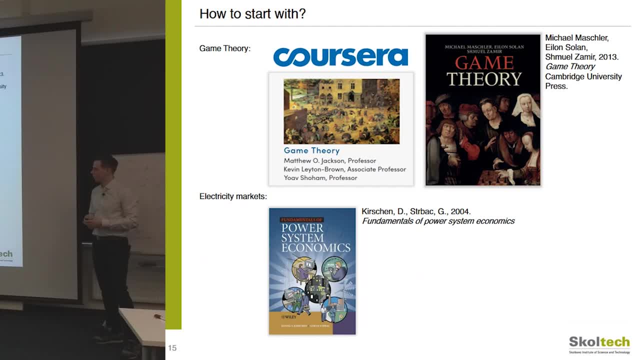 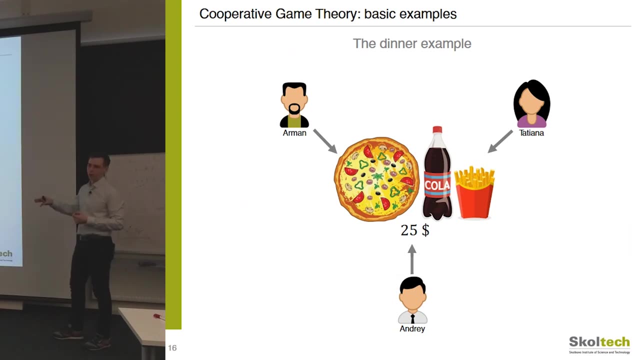 famous book that Janusz likes, Fundamentals of Power System Economics, And I hope that you are ready for more complicated examples once we introduce more players. And here I prepared for you the dinner example. And imagine there are three friends- I put just some random names like Arman, Andrei and Tatyana, and they discuss going to have a dinner, But for some reason they want to discuss this in detail. So I put some random names like Arman, Andrei and Tatyana, and they discuss going to have a dinner, But for some reason they want to discuss this in detail. 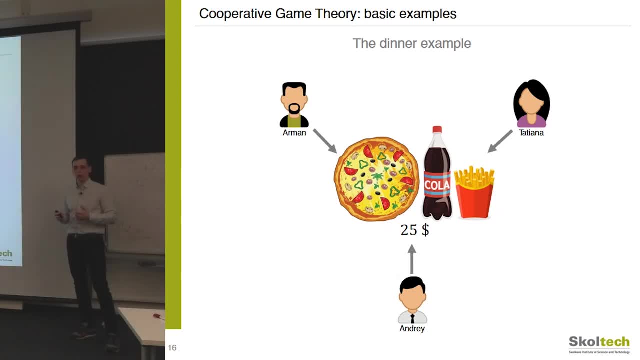 So I put some random names like Arman, Andrei and Tatyana, and they discuss going to have a dinner, But for some reason they want to discuss this in detail And they figured out that if they go together they will buy big pizza, cola and big fries. 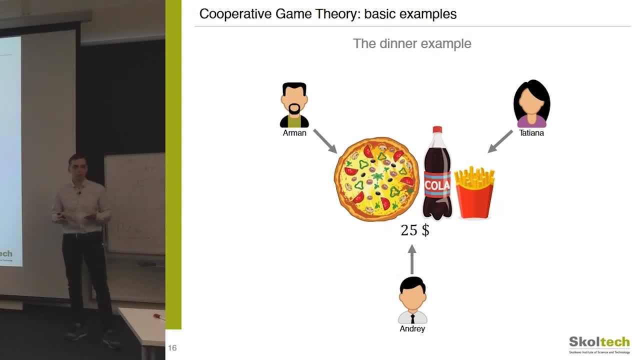 And the question is how they should pay for this. And in real life this question may be a bit stupid. They can pay in equal shares, or maybe one of the friends can say that I pay for all of you, But imagine that this is not a pizza but a multi-billion dollar project. 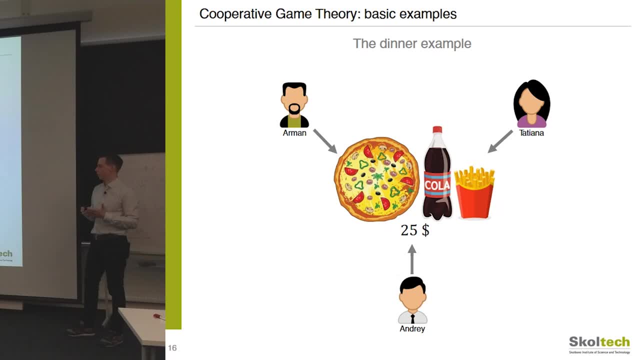 And this level of inaccuracy is unacceptable in such projects. So you need some justified solution for investment cost allocation And therefore we go to cooperative game theory And the theory tells us that you need to consider all possible scenarios of cooperation. And first of all, we ask people: what are you going to do if you do not cooperate today? 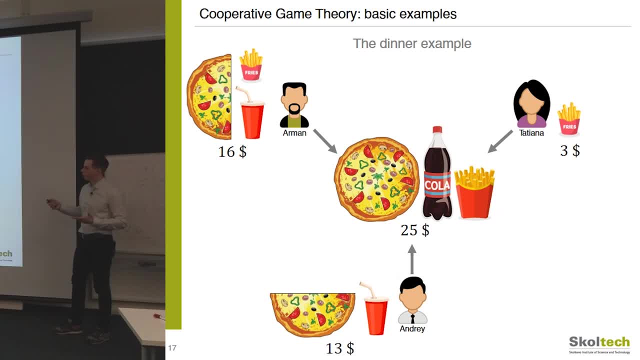 And we see that the players are in different conditions. For example, Arman is a bit hungry and he says: I am going to buy half pizza, cola and fries And this cost me $16.. Andrei is also a bit hungry. 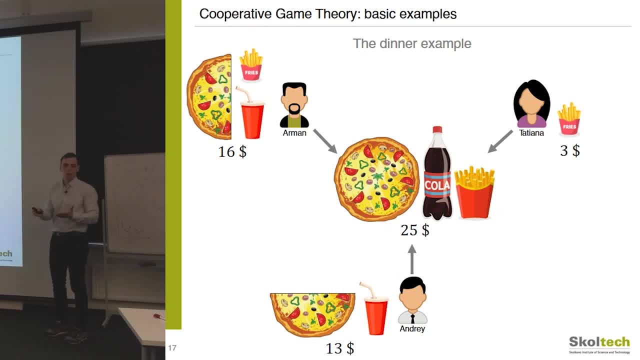 But Tatyana, for example, says: I'm just going with you for the dinner, But I'm not hungry, I want just small fries. So we see that they are in different initial conditions. But also, since there are three players, we need to consider more scenarios of their mutual. 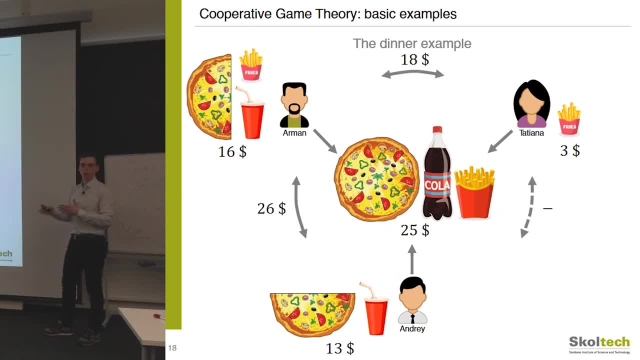 cooperation. What happens if Andrei goes with Arman but not with Tatyana? What happens if Arman goes with Tatyana? And maybe just for fun we can create a situation where Tatyana and Andrei for some reason, 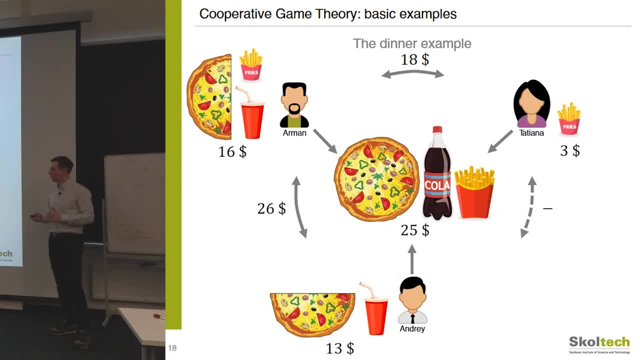 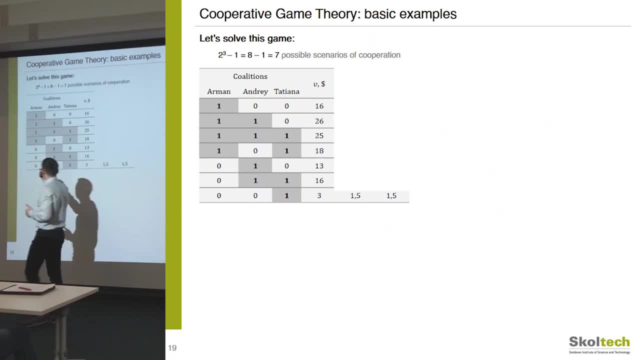 do not cooperate at all. They will not go for the dinner. And let's see what happens with this game. mathematically, We can create this table: And 2 to the power of 3 minus 1.. 4 to the power of 3 minus 1 leads to 7 possible scenarios of cooperation. 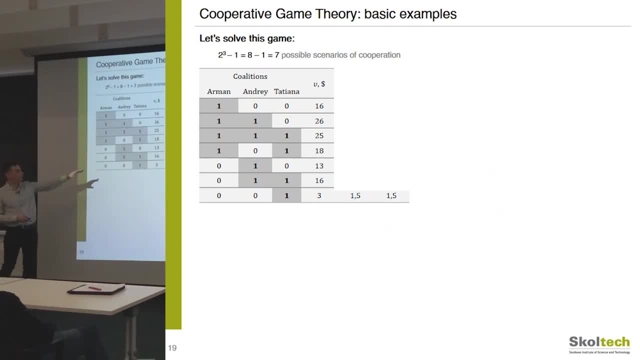 And you may see all the 7 collisions here- and the characteristic function, And based on this characteristic function, we can use the Shapley value formula and evaluate how the cost should be allocated among the players. And this is the Shapley value allocation. 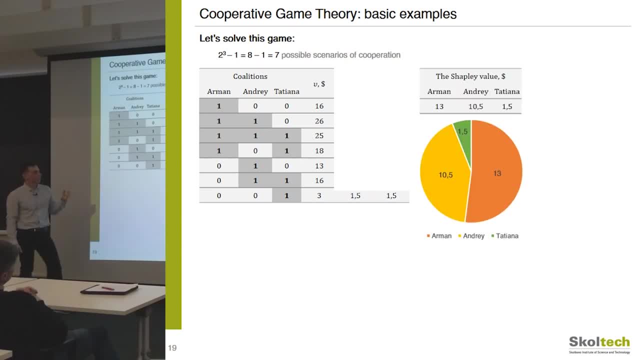 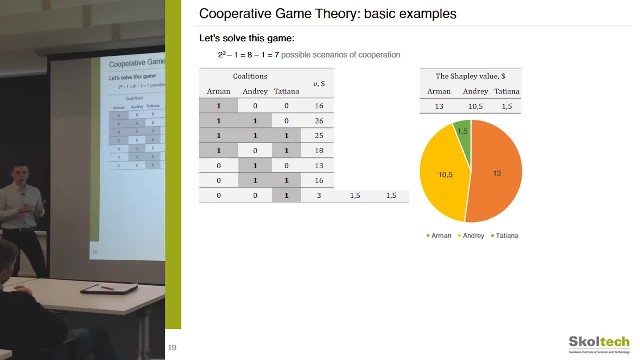 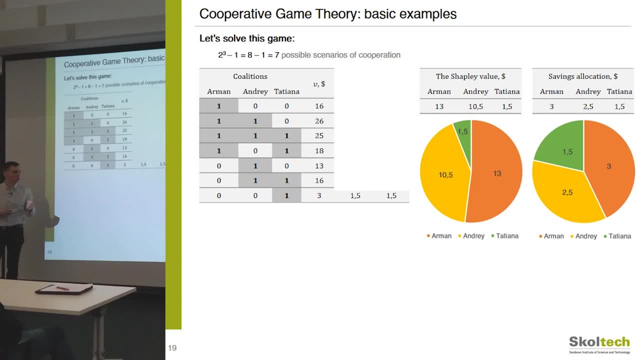 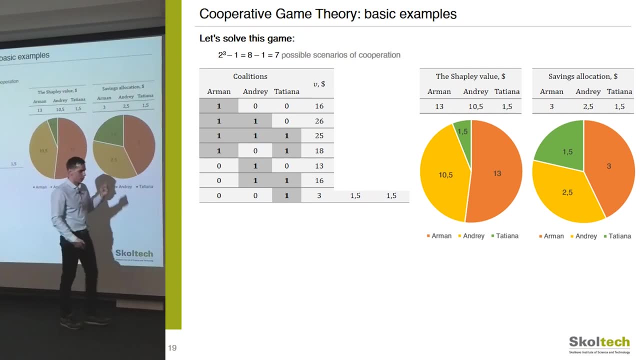 initial conditions and see the savings allocation, And the situation here is a bit different. The players are more equal, but still Arman has the better savings allocation and this means that he has a better bargaining power. in this example, He is a more influential player. 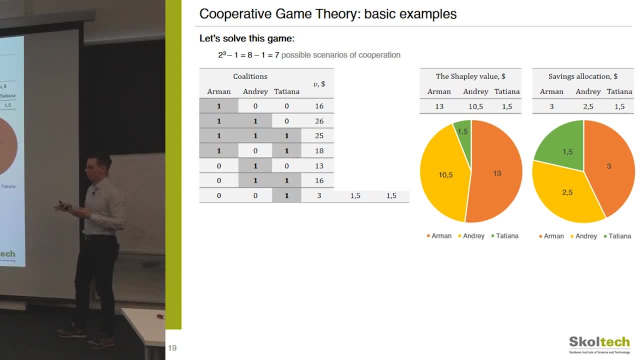 While Tatyana has not so much money to invest in this. she's not such an influential player, and this is just a. if you consider the savings as a ratio of the contribution, the situation is quite different. so tatiana now saves the most because she's about to invest three and she saves half. all right, if you, if you're saying percentage. 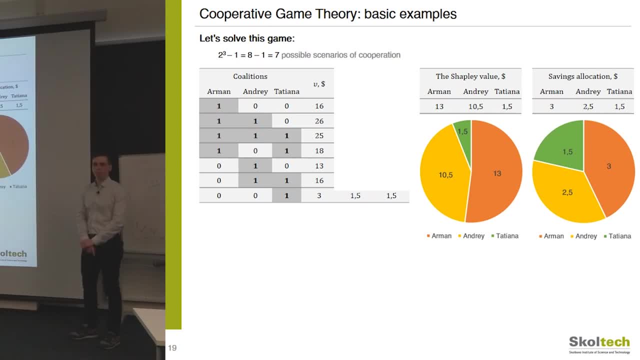 yeah, yeah, as percentage, her savings is much better, and it's the same in the other examples as well. i guess maybe, but if we consider, like in global shares, we see that armand gets gets more in dollars in terms of dollars, and this is just the, as i said, the most common solutions, and there is 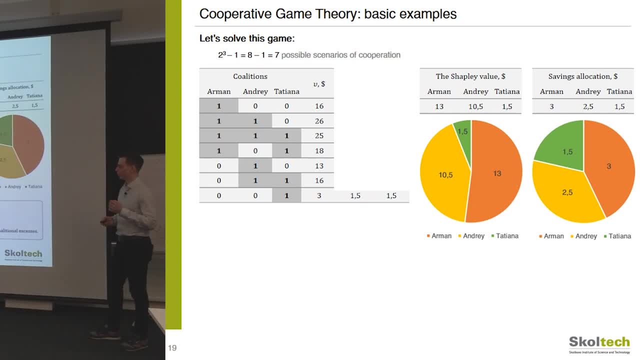 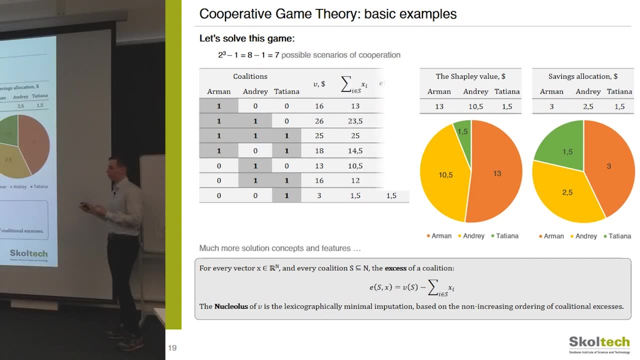 much more in cooperative game theory and i don't have time to explain everything, but just to give you some ideas. we can further, uh evaluate the solution that we got. for example, we can measure the so-called access of a coalition, and the access is the difference between what coalition. 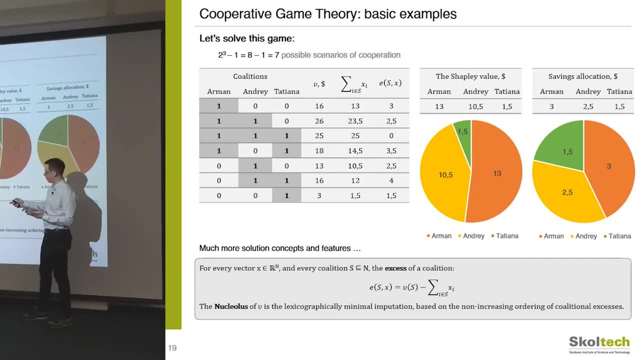 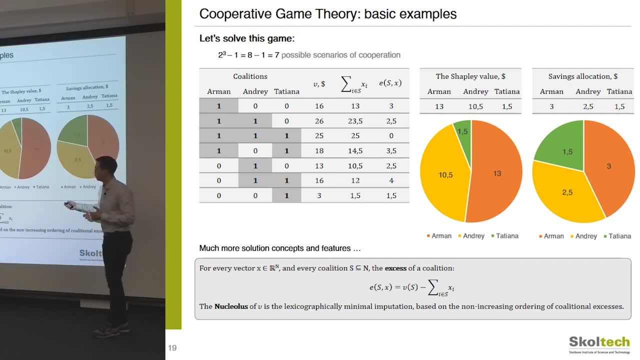 gets on its own minus what it is allocated, and therefore i created here uh additional column summarizing uh the sum of allocations for each of the coalition and the access. you may notice that for the grand coalition the access is zero because three players are three players there is. 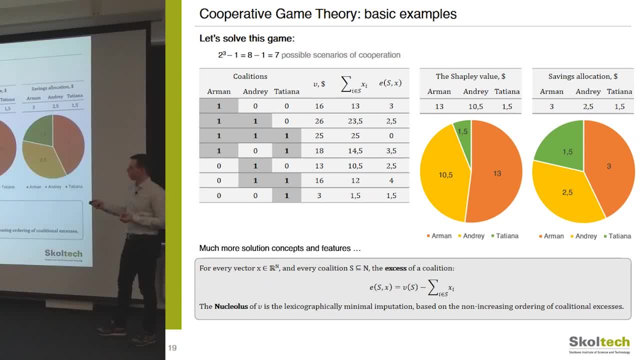 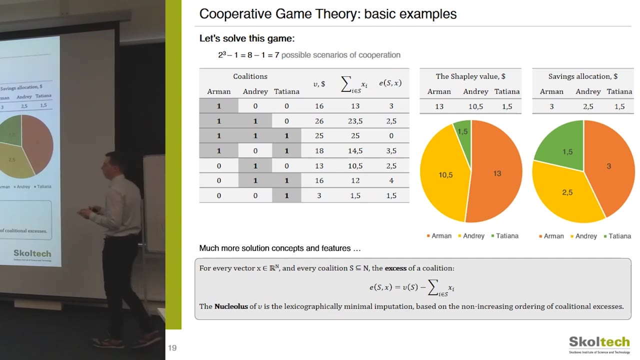 no difference and for other coalitions there there are some excesses and you may see that tatiana is the less less satisfied player because, as you said, in percentage maybe she goes a lot, but in terms of dollars she invests not so much and she, uh, she has not. so 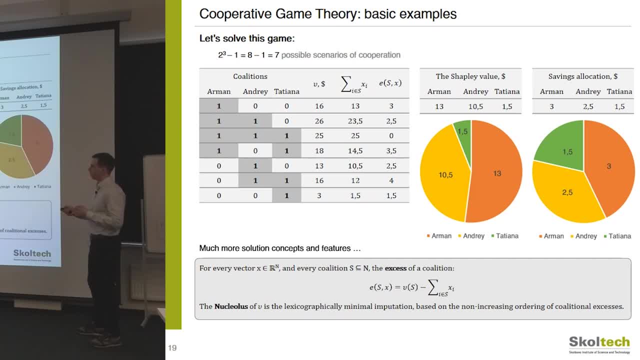 much surplus, and please notice that the most uh satisfied coalition is this coalition with the access for andre tatiana, because, yes, but you also do not consider that if two of them play together, they gain something. so, yeah, i consider this. yeah, so so you don't form a coalition, uh, of two in other. 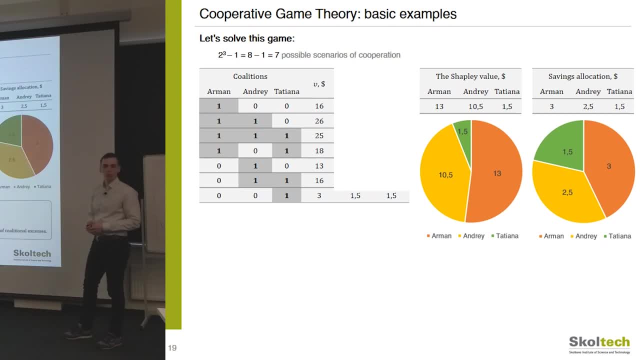 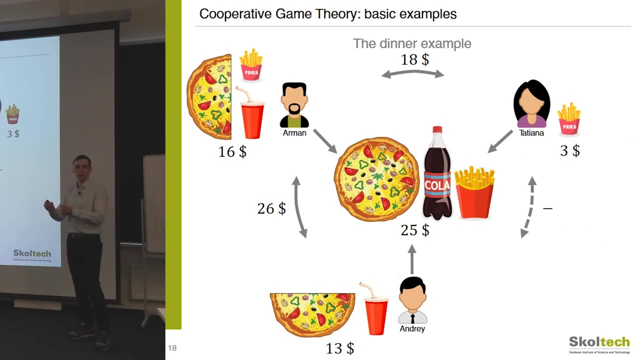 words, the, the, the coast for two is just the sum of their separate codes. no, i, i i created a game- uh, not, not to some. you may notice that this is not okay, so this is not the sum i created. this is called a super additive game when each coalition is better than no cooperation. 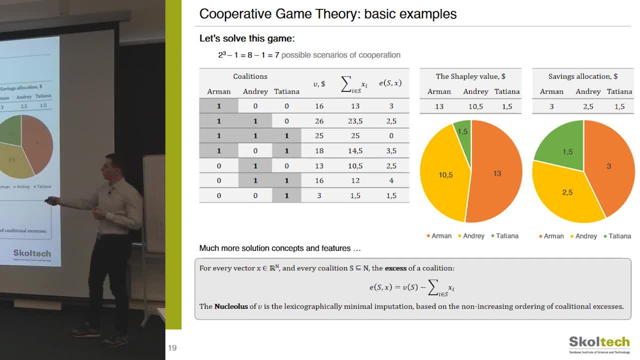 and yes, we, we can measure the access, we and this coalition. tatiana andre is the most satisfied one. why? because without the grand coalition they do not cooperate at all and once they enter the coalition with armand they get some surplus and therefore this turns out to be the most satisfied coalition. and, as i said there, 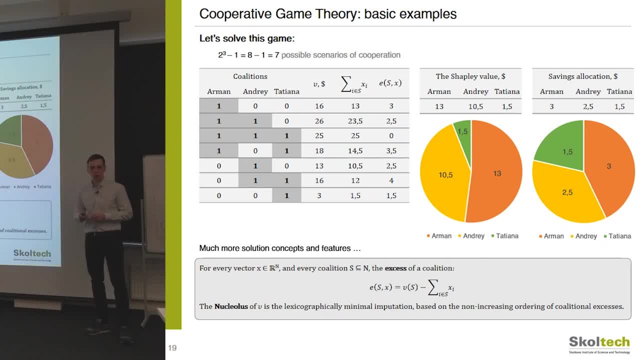 are much more solution concepts- maybe i will cover more details in the next lecture- and based on this idea of excess, there is a solution concept called nucleolus, and it is a series of linear optimization problems that tries to minimize the dissatisfaction of coalitions, and this is. this leads to rather interesting results, and the last example for today is the. 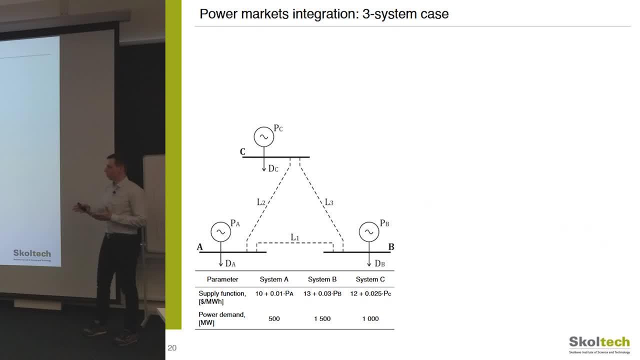 same three players, but in power systems. once again, imagine three power systems that are going to interconnect and i created different cost functions here, but still system b is the most expensive one and it has the highest power demand, and in order to solve this game, we need to launch the. 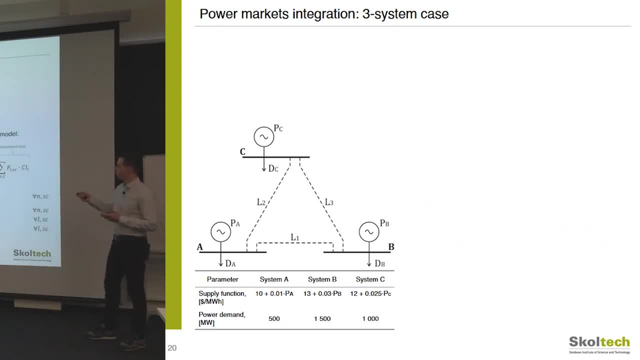 optimization model several times. so this is the same cost minimization model of generation cost and investment cost and we launch it for multiple scenarios. so let's see, this is scenario number one. i call this no cooperation. this is the generation cost. there are no lines, no investment cost and the total cost. 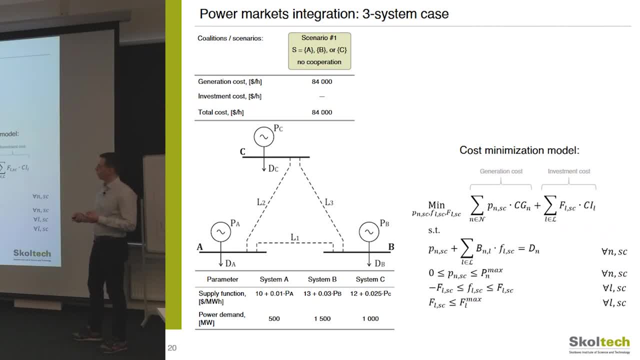 and then we start running optimization models. we calculate scenario of the grant coalition. you see that all the lines are built up to the maximum of 100 megawatts. then we consider scenario a- b. you see only this line exists: a- c and b- c. so we compose a characteristic function and we can implement the solution concepts. 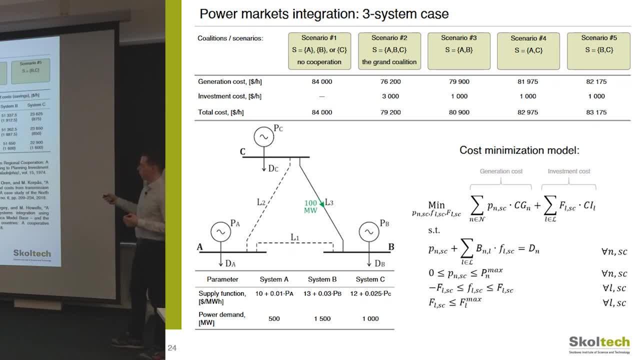 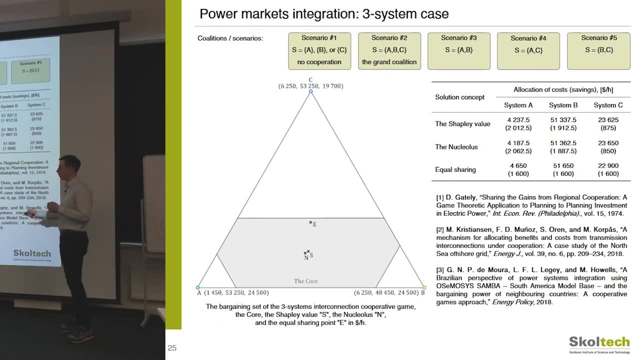 i show them in the table in terms of cost allocation and cost savings. so the shepley value, the nucleolus and equal sharing. and, more interestingly, there is a way of plotting this using this barycentric coordinate system. and in order to give you an idea, what is barycentric? 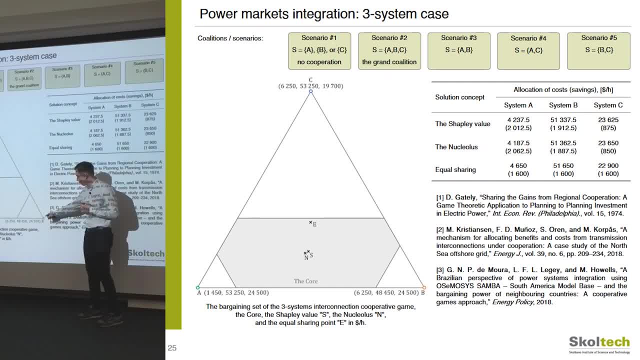 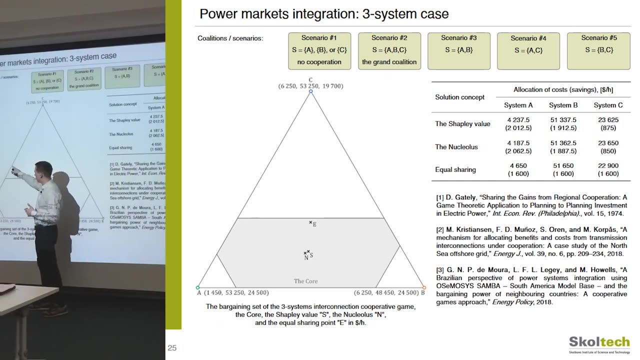 coordinate system. you may consider point b, and this is the point where system b gets 100 percent of savings, and the further we move away from point b, system b gets less and less savings. this means that here system b gets zero savings, and this is an interesting way of showing the possible. 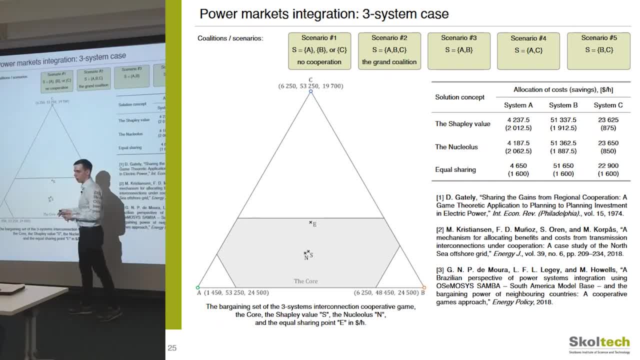 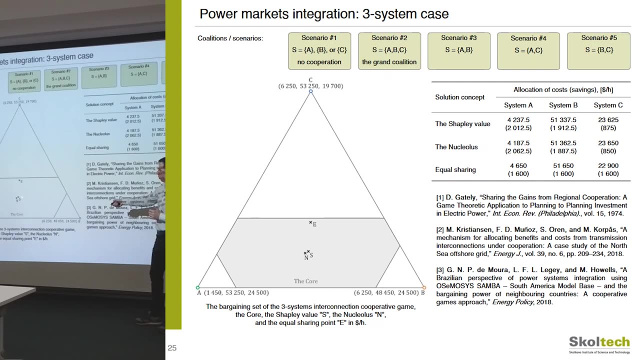 allocation solutions and this region inside is called the core of the game. as i said, the convex set formed by half spaces and some interesting solutions. for example, right in the center of mass of this triangle we have the equal sharing point, one of the most obvious solutions, and shepley value and nucleolus. they're rather close for this case, but we see that. 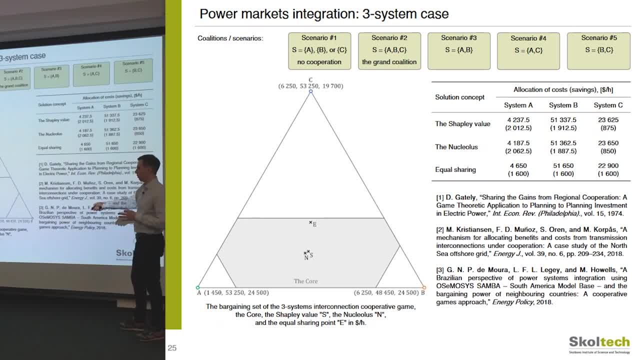 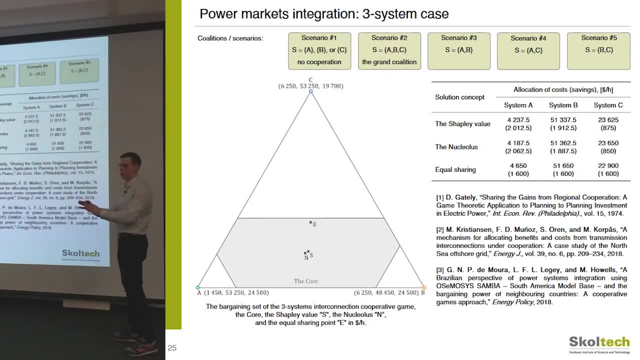 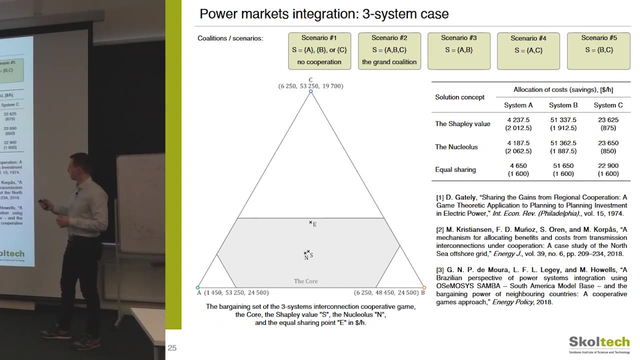 nucleolus sees that probably player a is a bit underestimated by the shepley value. so the allocation solution moves a bit towards system a and this approach has been implemented many times. i found several papers started from a famous paper by dermot gately in 1974 and some modern research about 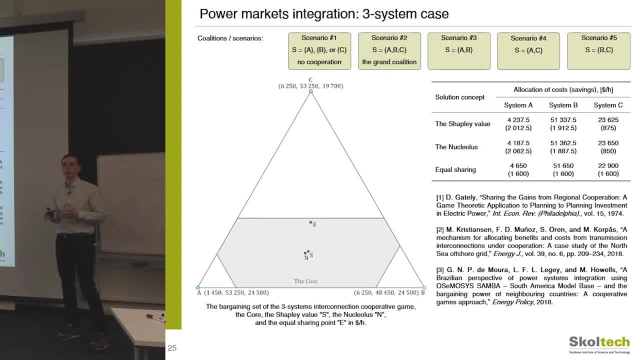 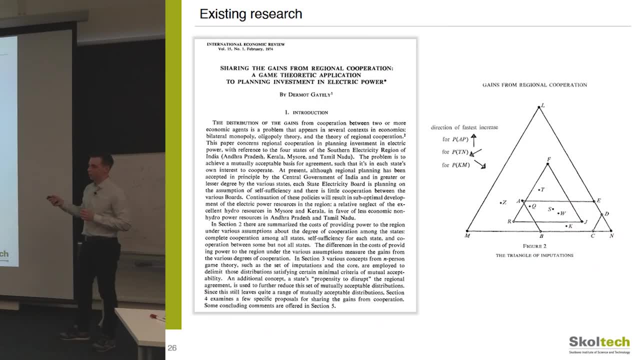 interconnections in the north sea and interconnections among brazil and its neighboring countries. and just to show you some of the research, this is the famous paper by dermot gately and i think it is amazing that this research was done more than 40 years ago without computers. he plotted such a nice graphs, also visualizing possible allocation. 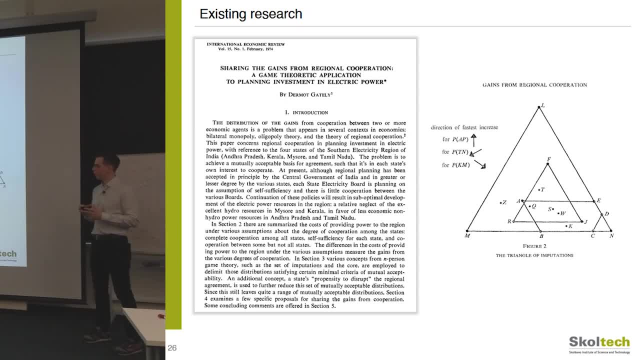 solutions. he considered three power systems in india as a case study and he considered many the nucleolus. he also suggested his own solution concept that he called propensity to disrupt. and then the next influential study that i know is the study by javier contreras in 1999. by the way, this 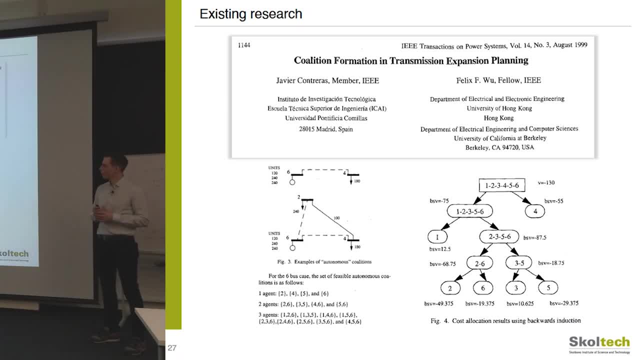 is the supervisor of professor david pozo and he also considered possible cost allocations and coalitional formation in power systems and, as you may see here, he used a backwards induction to consider how the grand coalition formed and the the whole history of formation, and used this to 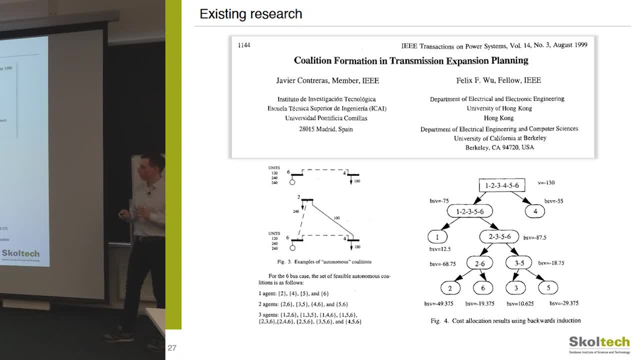 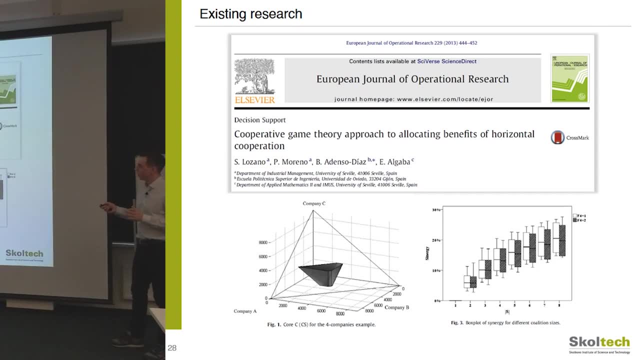 allocate the costs among the power systems. and there are much more papers. just to give you an example, there is a paper not about power system but about so-called horizontal cooperation, and lazana here explained how horizontal means more or less equal firms at the same level of operation. 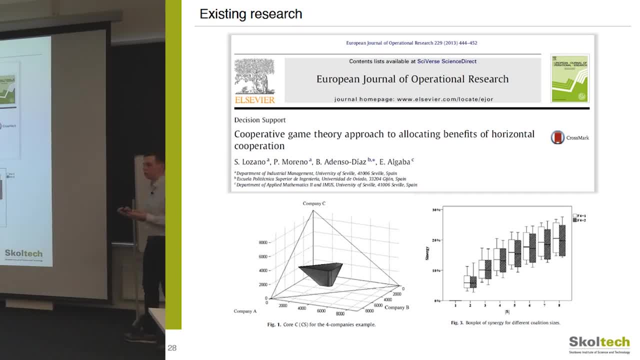 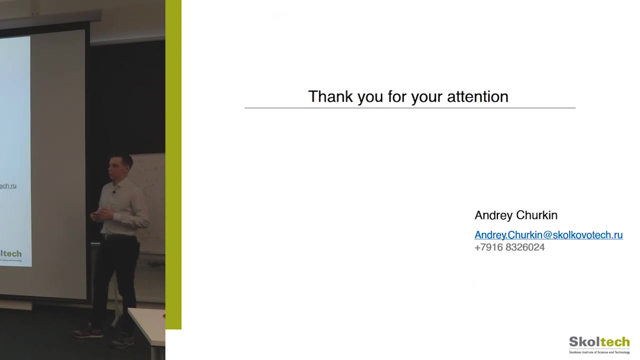 can cooperate to get some synergy, and he explained this on the basis of logistic costs for shipping, how the shipping companies may cooperate to get less cost. and also, you may see that he analyzed the core and different solution allocations and he concluded that this could be implemented in many, many applied topics. so, yes, i think that's all for. 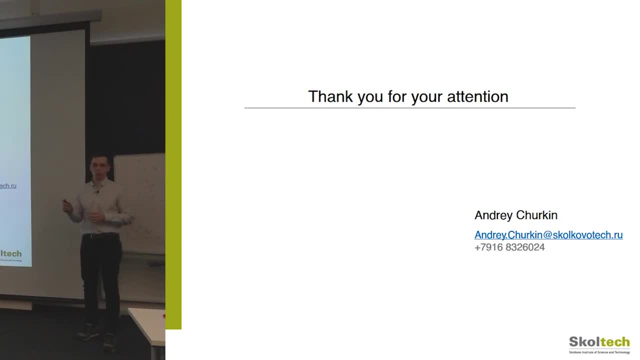 today and i want to tell you that in this is not the only way to implement cooperative game theory in power systems. i saw papers about cooperation of microgrease, when they agree of building some equipment or following some rules and then they share the allocations, or cooperation in co2. 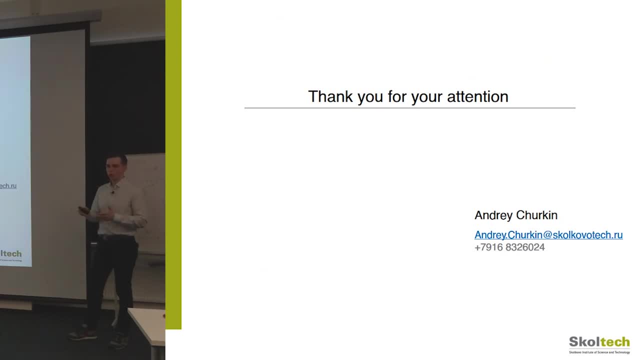 emissions reduction. so there are multiple ways when you can think about how to implement cooperative game theory and it will give you some insights about players position in this cooperation and possible ways of transferring money and so on. so i hope you enjoyed this lecture and thank you for. 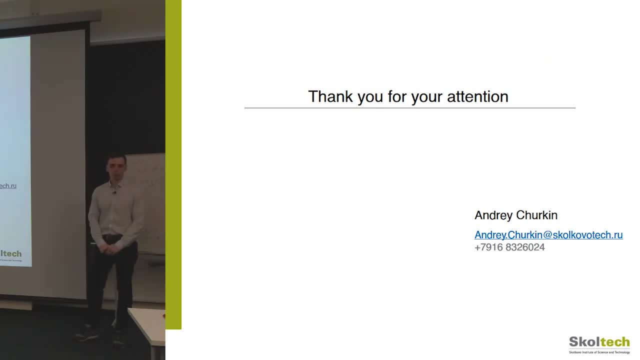 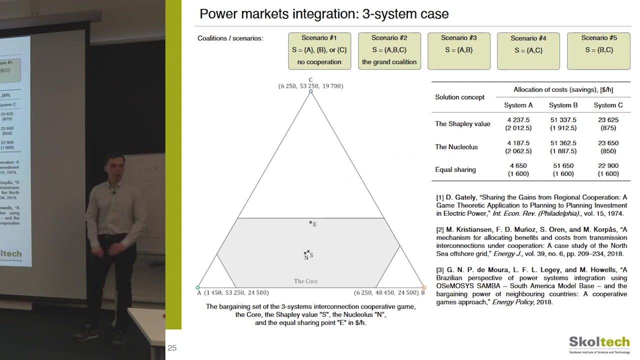 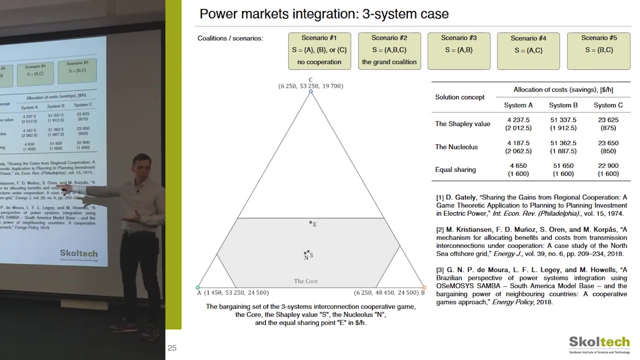 your attention. yes, uh, this point where sharply you understand equal sharing is this point. does this point correspond in some geometrical or physical property of triangle? yes, a center of mass is equally distant from right. equal equal sharing point is the center of mass. yes, and therefore yes. 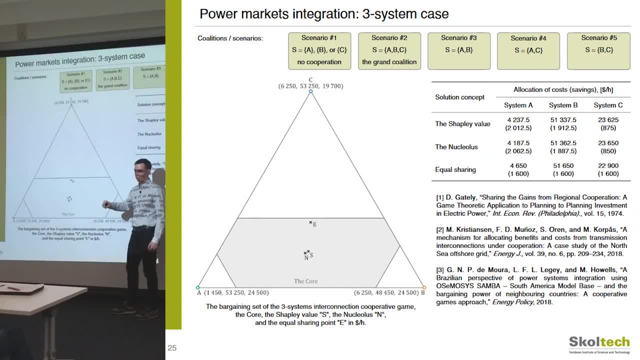 and below. uh, there is. there are some interpretations, but they involve game theory. but basically there are some sets and you try to find a weighted average of of this set. this is called the weber set, if i'm not mistaken. this is similar to the core, but it's a bit a bit larger. 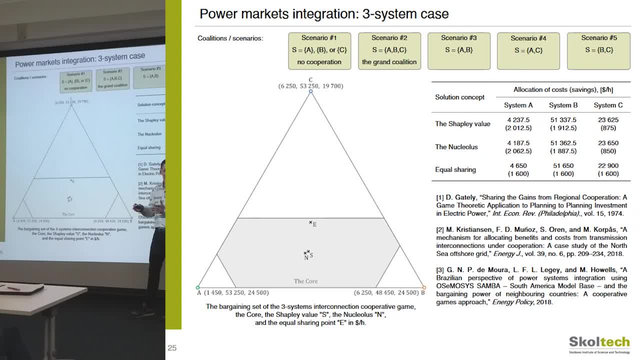 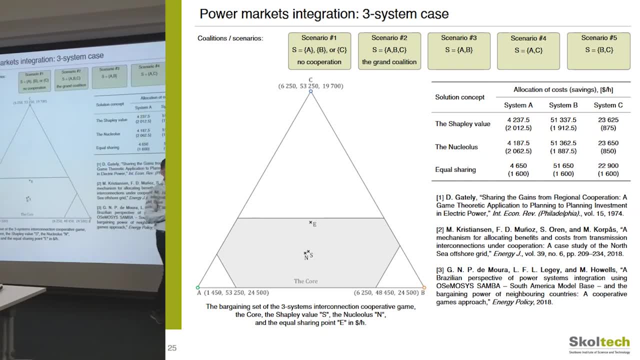 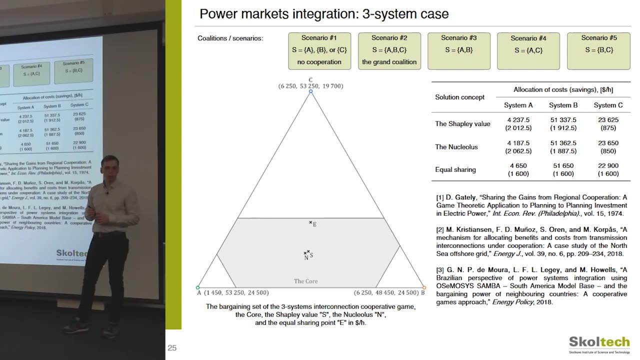 so you, you find some weighted sum of contributions, yes, like shapley value does, and you find these final points and you can plot this as you see, as you saw, even in 3d: yeah, also nucleolus have some correspondence with the core right. yes, nucleolus, it is proven. there are many theorems in game. 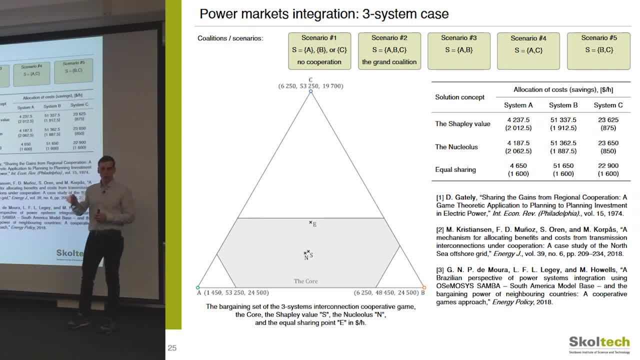 theory and, for example, it's proven that if the core exists, nucleolus is always the part of the core, so it it's somewhere in the middle. so if you- okay, indeed, if you consider like equal, then the mass at each point a, b and c is the same. 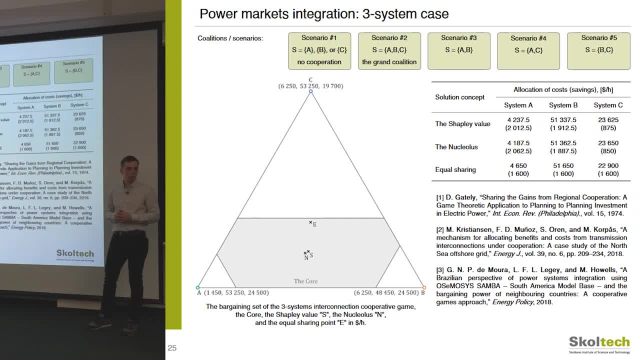 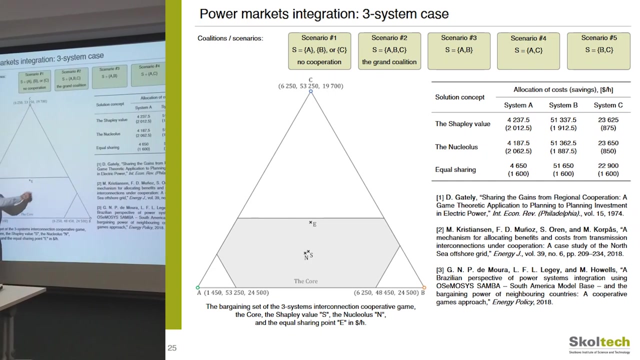 and then the, then you're exceeding the center. but what if? so you have different combinations when the masses associated to points a, b, c and c are different. right, if, if, if players are in equal conditions- initial conditions, you will see. if that there will be the core like a triangle, somewhere like perfectly centered. but you see that this feasible space 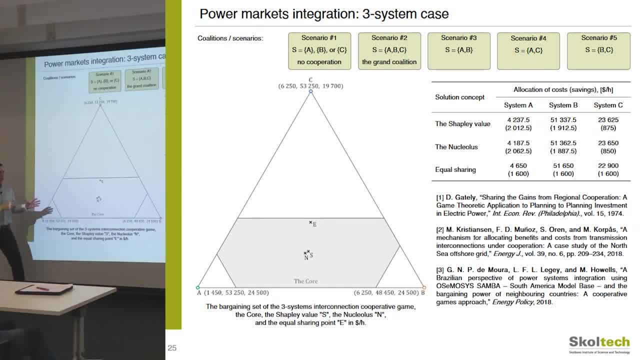 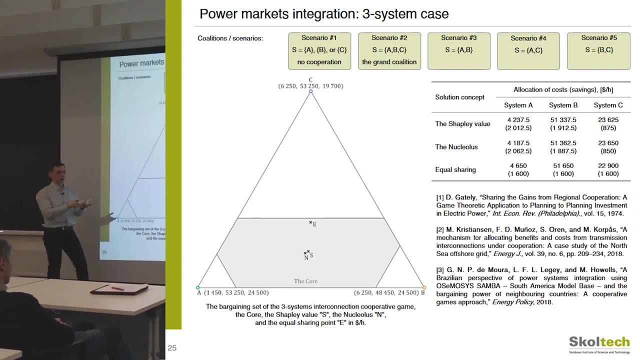 shifted towards system b and and a, and this represents the inequality that this figure, like triangle itself, stays the same, but the core and the solution moves inside and if, if some system is more influential, probably the location will move towards it, it will get more, so the point and the core moves, but the, the figure stays the same. 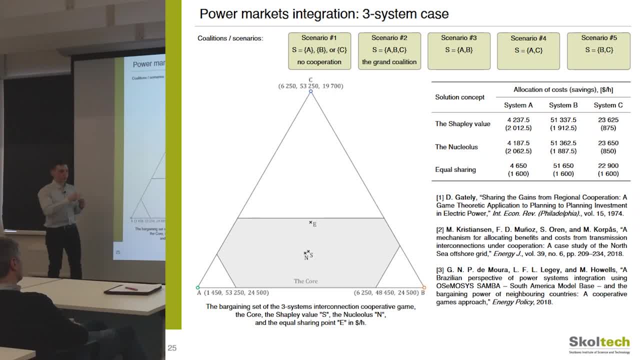 it can. it can enlarge or shrink. if you allow to build more lines the whole triangle, this space can just expand. or if you forbid the lines, there will be zero space, like no cooperation. can you go back to the figure with the areas red and blue that you have between only two areas, 400? 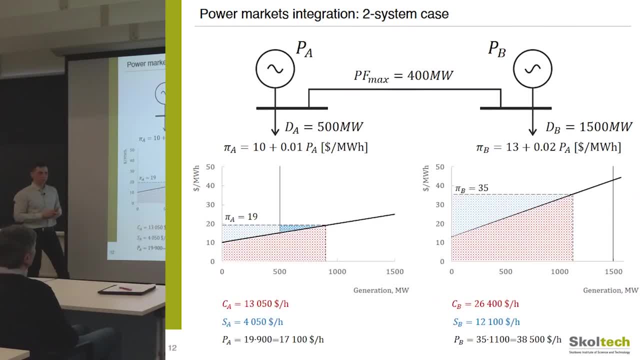 megawatt interconnections. so basically, when they interconnect, i mean you solve an optimization problem and you derive what is the? basically the direction of the flow and the total cost of the system. yes, right, and you also have, like, let's say, a cost for the area a and the cost for the area b, right, yes, and those? 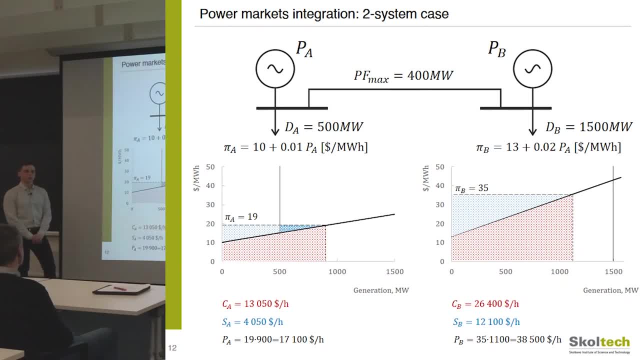 costs are going to be, uh, let's say, different than the ones? if they are, yes, okay, what is the, let's say the motivation of the area, that is, reducing the cost of using the sharply value to calculate a new cost allocation, then okay, so the initial cost of area a was really low. 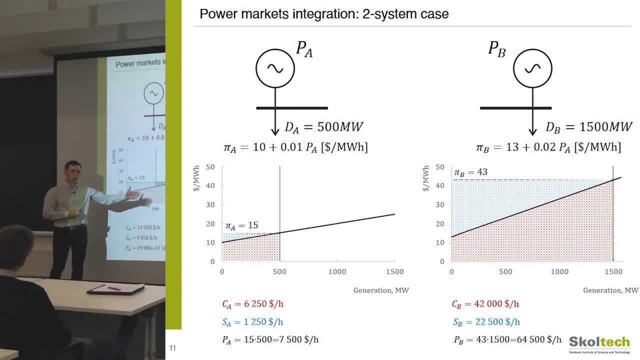 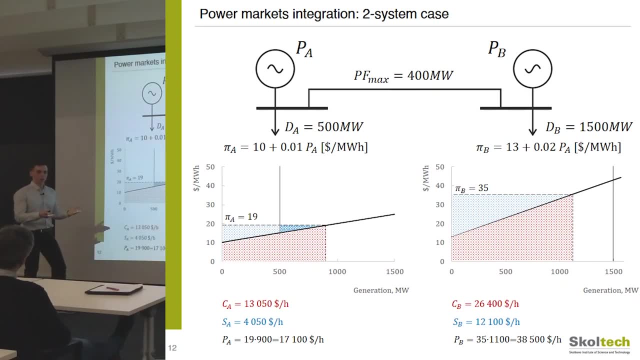 and then it starts exporting power and basically it suffers because it needs to generate more. so it needs to be compensated somehow, and in this example you've seen that there is enough savings, enough money on the table to compensate it, because the sum of generation costs here is larger than the sum of generation costs in the interconnection scenario. 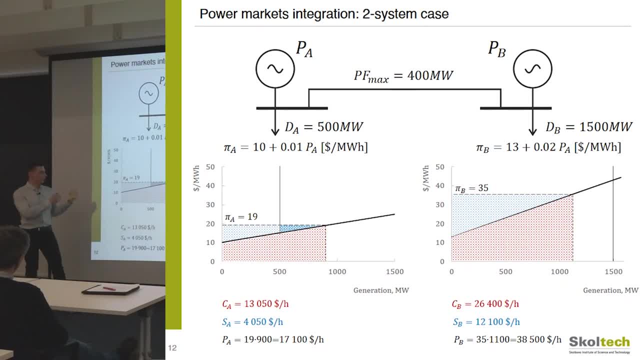 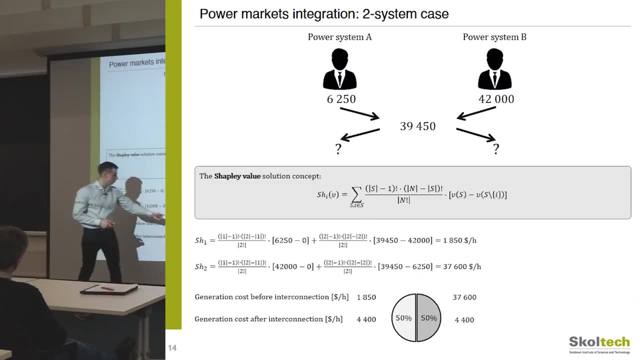 and the question is: how much should system B pay to system A? and this can be calculated based on the Shapley value, that we get these allocations and we know that system A should end up in this point in having this cost and therefore we can calculate, okay, how much should be transferred. 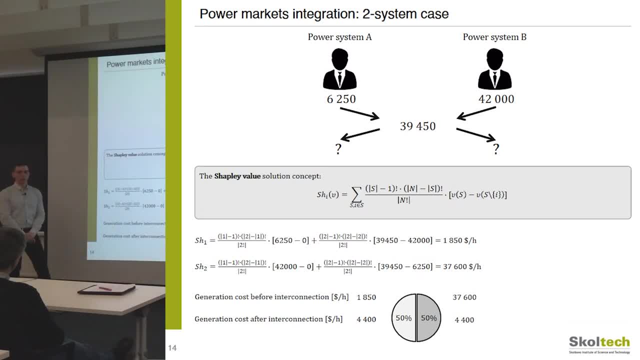 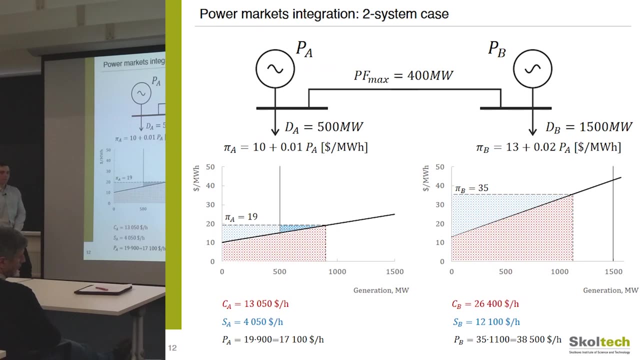 so this is one of the ideas, how to calculate this compensation. but does that diverge from the? if you go to the previous figure? so I have a locational marginal price on A and on B, right? so basically, if I have the locational marginal price on A, 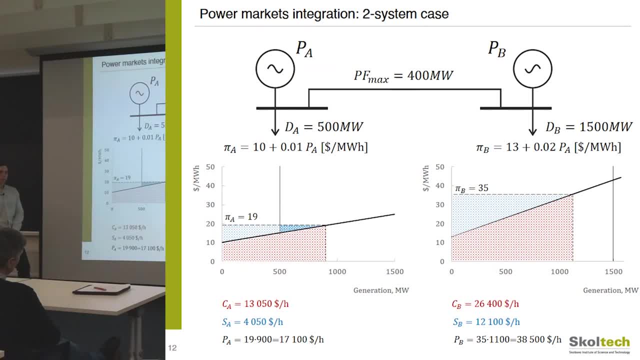 I just multiply that by 400 and I would have how much B would pay. does that differ from the Shapley value? no, this is direct from optimization and from energy economics. yeah, you see it. the prices are also plotted here. they change: this price increase, this price, those price decrease. 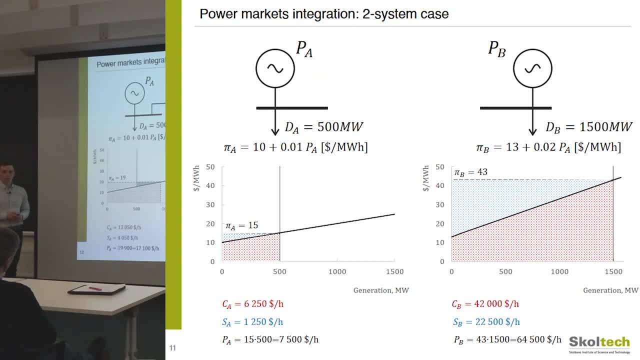 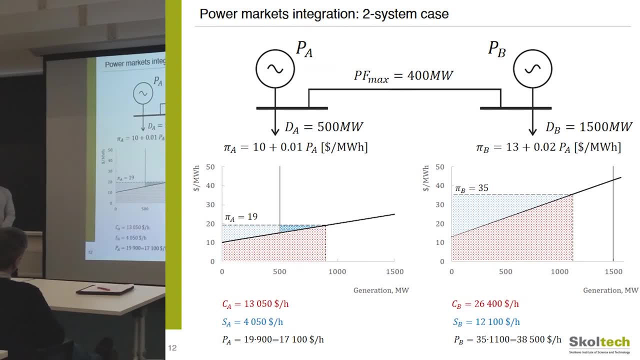 so I'm saying that your solution will exactly correspond to the locational marginal prices? no, because the location prices, the marginal prices, they will depend on whether the line is congested or not. so it's congested in your case. yes, so we will have some solution. 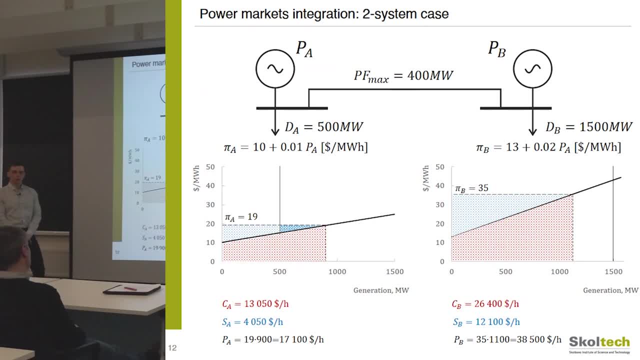 there is still a difference. yeah, yeah, of course you will have some solution and it's not the solution that you just presented. it's different one. based on the locational marginal price theory, I can evaluate what would be the cost, the prices, but if there is need for compensation, we can turn our attention to cooperative game theory. 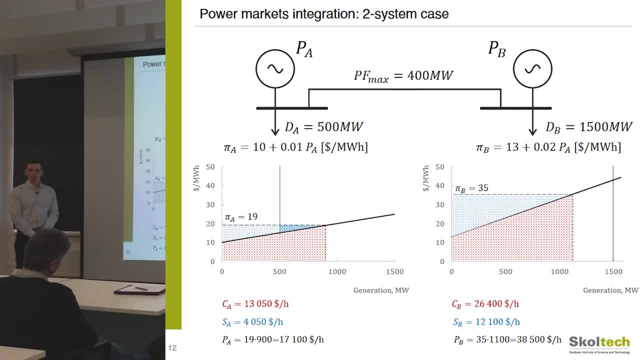 but you see, when you've got the location- marginal prices- you kind of calculate the compensation automatically. yeah, don't you? not? exactly because there are many players and generators here will be happy to export more power because the social welfare increase, but yeah, but the consumers will suffer and maybe they will not agree to cooperate. 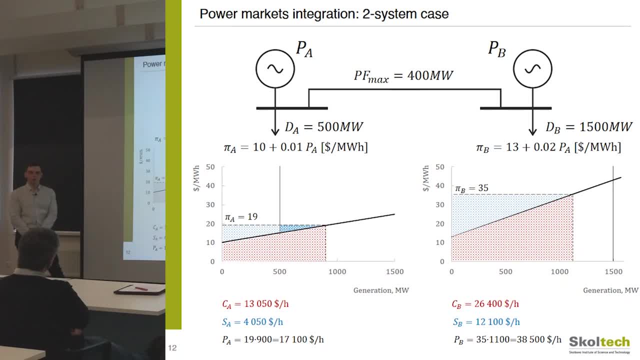 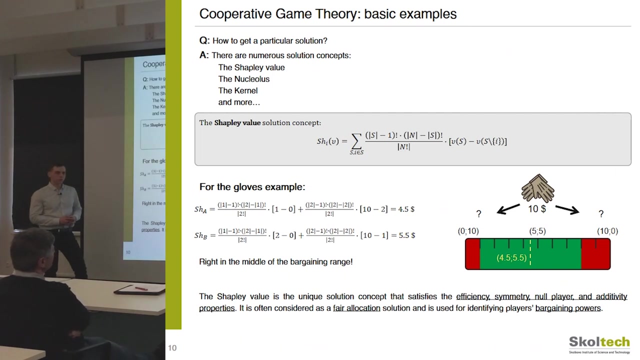 so there are multiple parties to be compensated. okay, we look at Shapley. can you show this? yes, Shapley value: yes, and these conclusions are failed for deterministic case when we are strictly determined. I can strictly determine characteristic function: nu, nu, yes, for each collision. 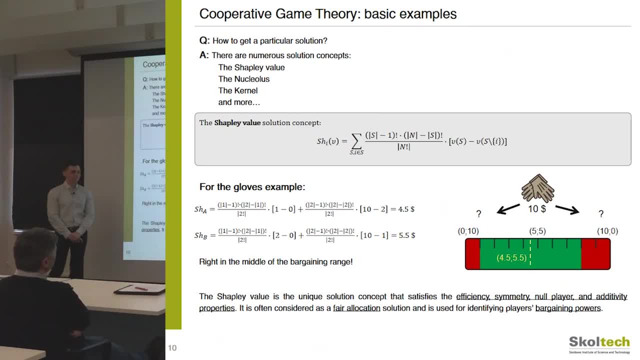 these conclusions are conserved for case when nu of s are nu of s have some uncertainty, for example, some noise. I saw at least one paper when they said that what if we don't know what is the value of collision? we only have some probability. and it is much more complicated. and people did this. they put probabilities inside. 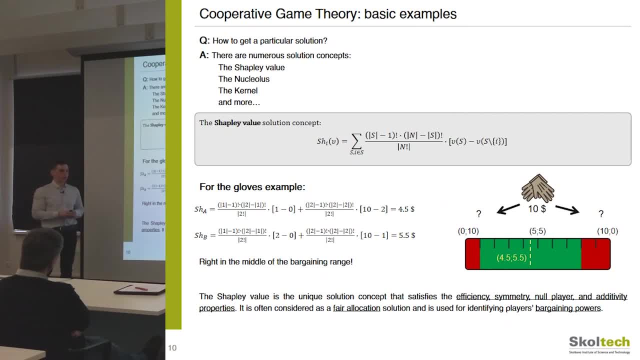 it is possible. I didn't do this, but yeah, if you don't have any deterministic data, you can make it more hard. but yeah, this example is. this example is static, one deterministic. you mentioned fairness a couple of times, so how to measure, like how fair some solution is? 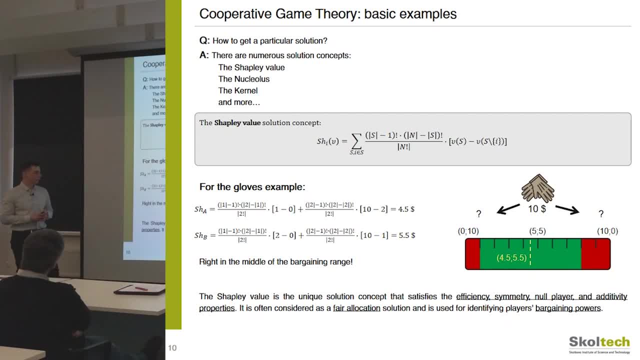 it is. it is a hard question. there are- there are many- how to say many- definitions of what fair solution should satisfy, and in this slide I mentioned the efficiency, the symmetry, the null player. and there are much more theorems and, for example, efficiency means that it, the entire value, is distributed fully. 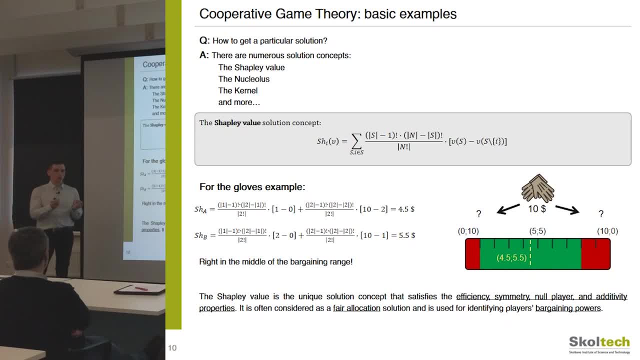 the symmetry means that if there are two players in exactly similar conditions that they will get exactly similar like equal payoffs. the null player is the rule that if player brings nothing he will get nothing eventually at the end of the allocation procedure and much more. and Shapley value satisfied satisfies a lot of these properties and therefore it is said that it is more or less the same as the previous one. 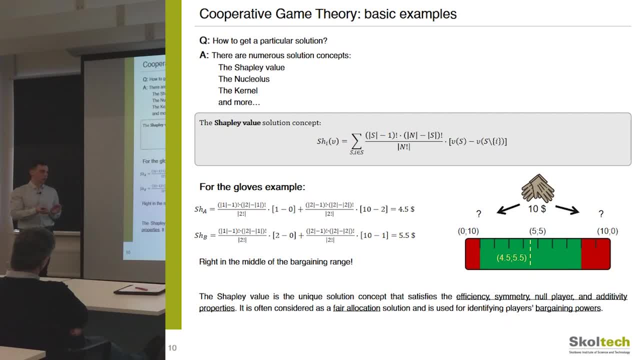 and therefore it is said that it is more or less fair solution where, while nucleus can allocate something, maybe two players, who brings almost nothing, and some properties will be ruined. but this is not. this is not so obvious. even to me, some of these definitions are not obvious. 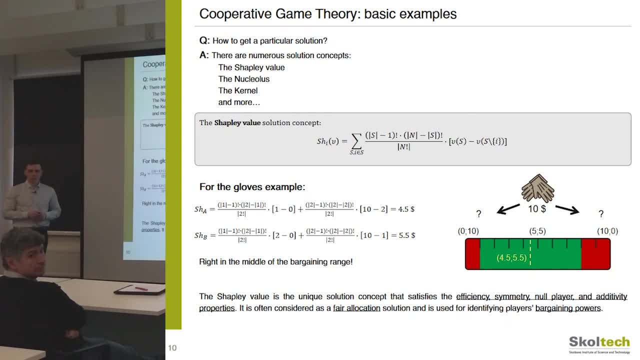 I feel like the concept of fairness is related with a marginal value, so, like, when you see a, when you see a, when you have the option to cooperate, you can understand what will be the marginal value. and so, for example, if we are operating number three like the sample of the table was really nice, I think. 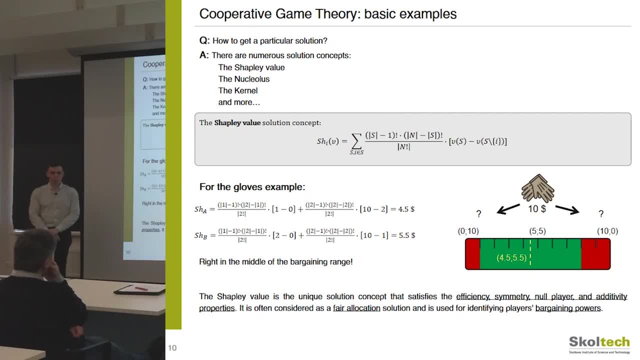 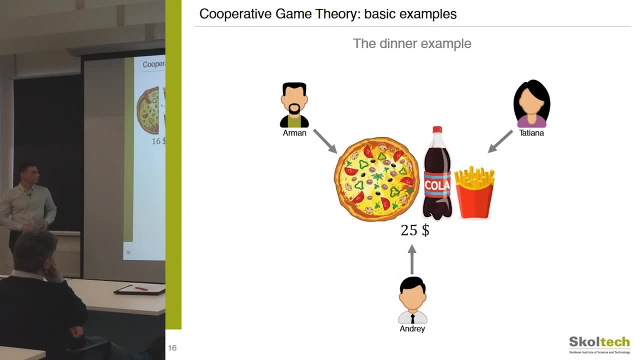 because we can think like well, two of us we are trying to pull up the table, but we were not able. but then Peter come and then they pull up. so his marginal contribution actually was a lot, was for us was zero and with him was one right, so we pull up. but this is not fair to give him like all the credit. 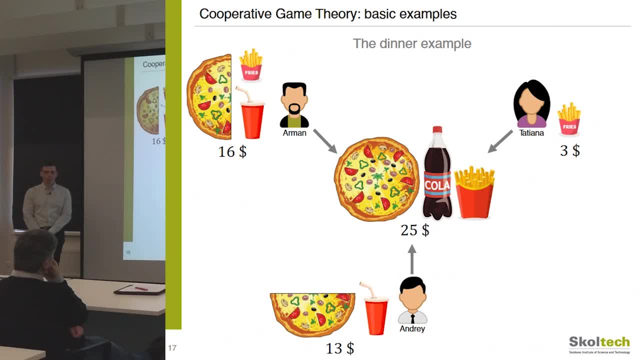 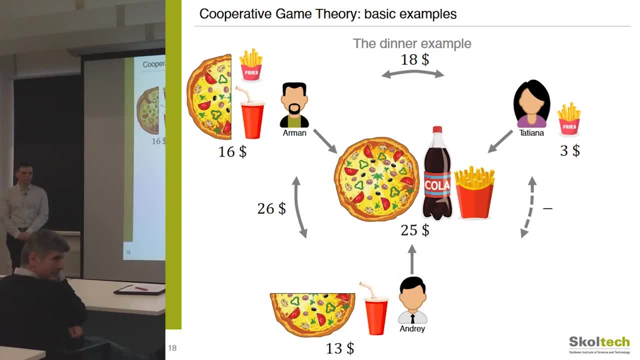 then there is this concept of creating all these possible- yeah, all the possible- combination, how the cooperation can be generated. so then, so we make the assumption, like Peter and myself, so we are trying to pull up the table, and then so this is another scenario, so those scenarios that he was mentioning. 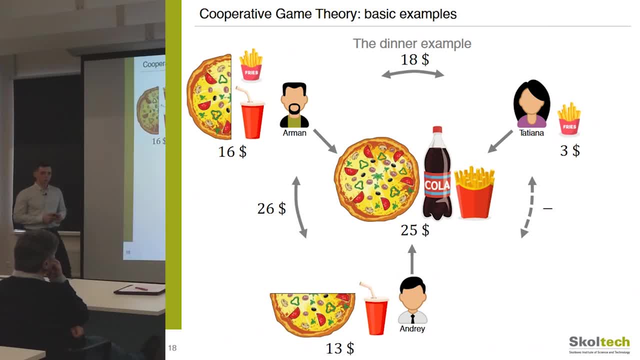 so at the end, so you can see like there are a lot of possible combinations that actually create some benefits. So you can see like there are a lot of possible combinations that actually create some benefits. So you can see like there are a lot of possible combinations that actually create some benefits. 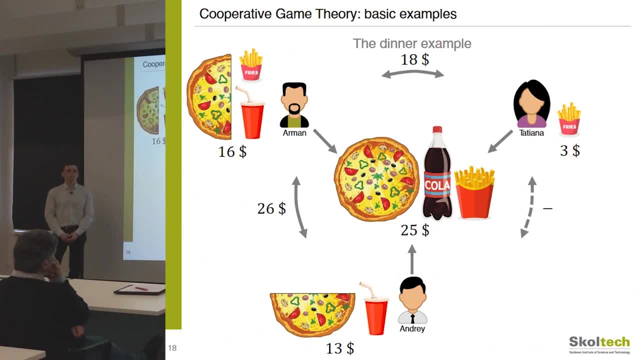 of value. oh, you have to compute what is this marginal value? And you have to compute what is this marginal value for Eureoce's situation? and there is this. There's a monster there on the beginning of the check-in value, but this is not really the proportion. 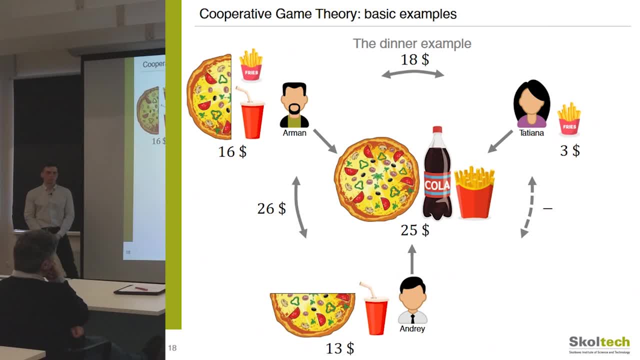 or like: what is the probability of having this in that right or or the combination so, fairly fashion, is that a sabi value? is that the only allocation rule? they give you fairness? and this is not because, also, I think you probably gave something you totally talk about: how does this really work?